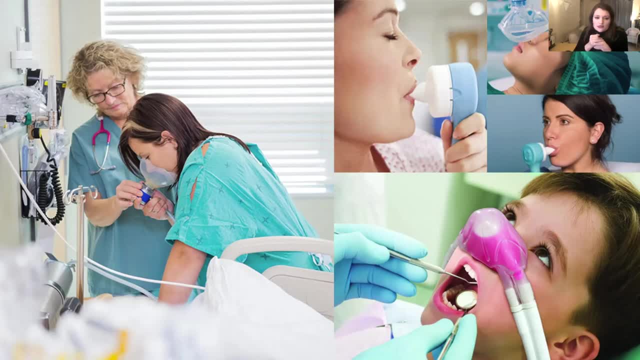 our disciplines. We want our patients to be able to use this medicine without their care being compromised, and we want our staff to work in a safe environment where they are not put at risk by nitrous oxide being present where it shouldn't be. Why should we be concerned about leakages, then? 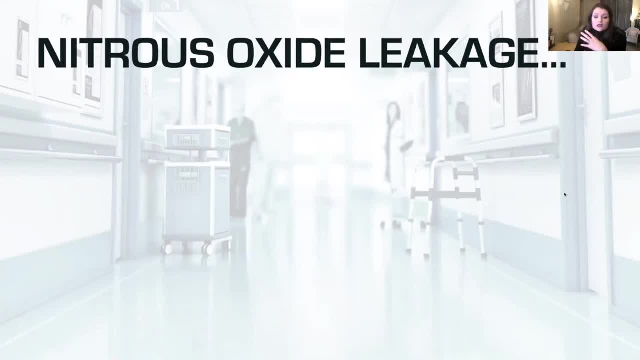 It's important for our hospital hallways, our rooms and actually for our bodies too. Nitrous oxide is regulated under COSH. it's a substance hazardous to health. It has an occupational exposure limit of 100 parts per million over an eight hour time-weighted limit. 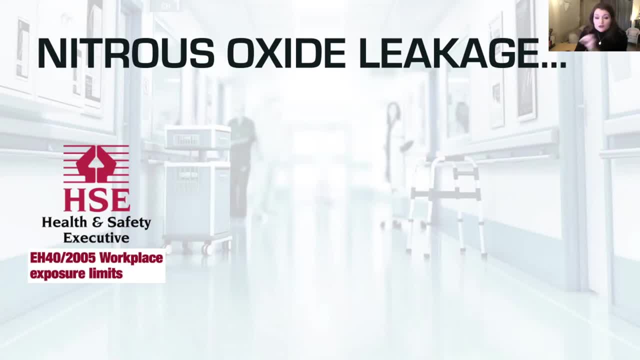 and that's in the UK, compared to 25 parts per million in Australia and the US. Nitrous oxide products are responsible for at least 75% of the anaesthetic gas footprint, which is important when considering the work that we've already started on volatile gases. Nitrous oxide is associated with 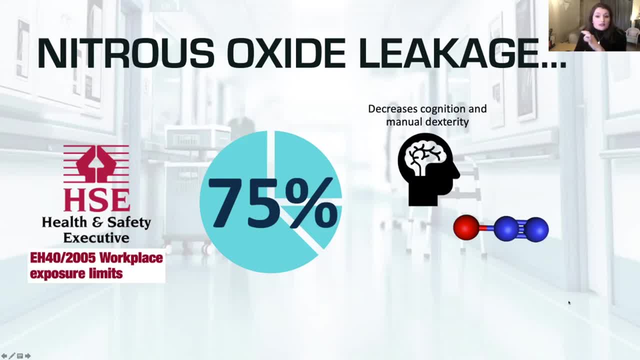 immediate-to-permanent and immediate-to-permanent use of nitrous oxide. Nitrous oxide is associated with immediate-to-permanent and chronic adverse physiological effects. It decreases cognition and manual dexterity. it's linked to vitamin B12 deficiency. there's an increased risk of miscarriage and adverse 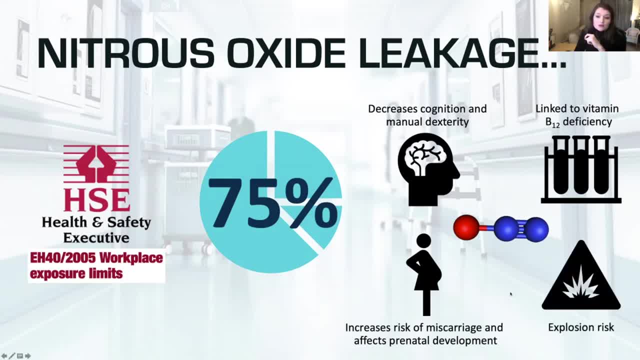 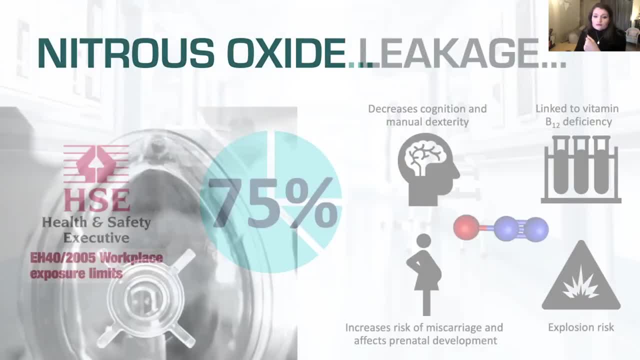 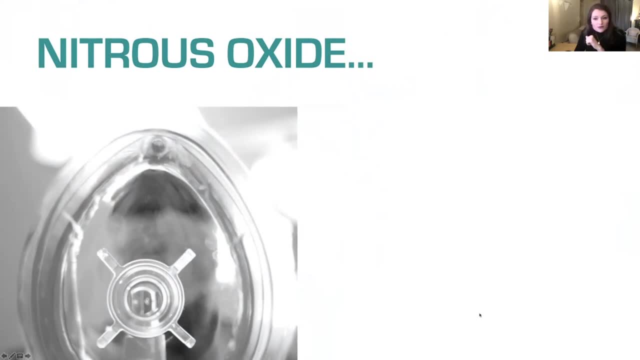 prenatal development and nitrous oxide decomposition has led to large tank explosions and, obviously, mixed with oxygen, is highly flammable. Why should we be concerned about leakages on a global level? What are the confirmed facts? Nitrous oxide is a powerful climate pollutant, over 250 times more damaging than straight up carbon dioxide. so it heats up the 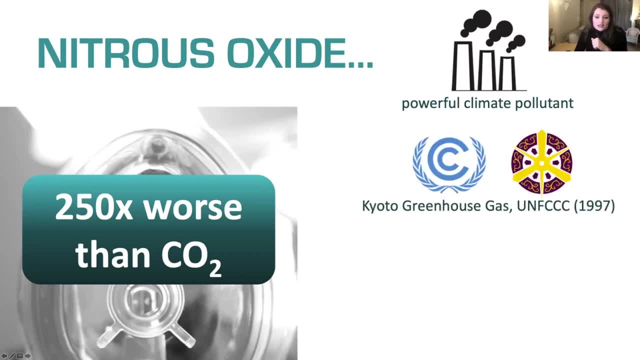 planet 250 times faster. It's one of the six major greenhouse gases named in the Kyoto Protocol, an international agreement by the United Nations Framework Convention on Climate Change to monitor and reduce emissions of said gases, an agreement to which the UK has made binding commitments. 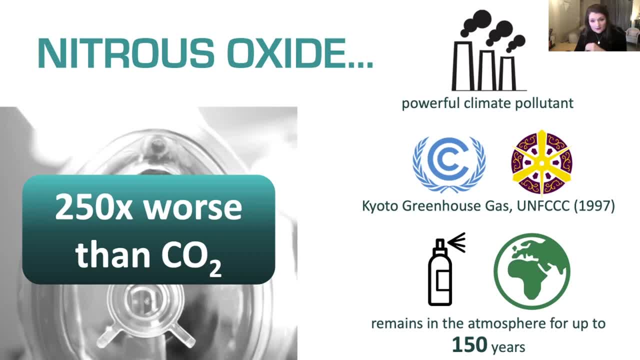 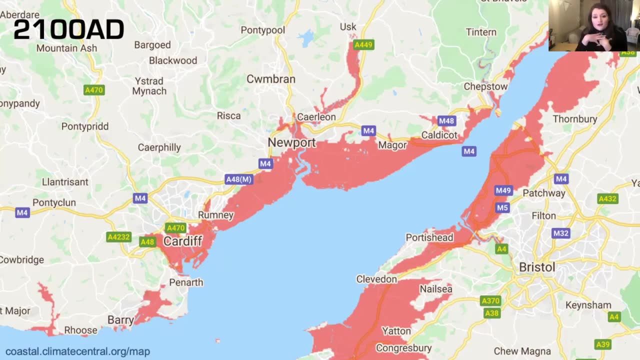 Nitrous oxide remains in the atmosphere for up to 150 years and it's known as the tangible successor the CFCs that destroyed the ozone layer towards the end of the last century. Now we can extend our thinking further, to the future picture. I find this shocking. 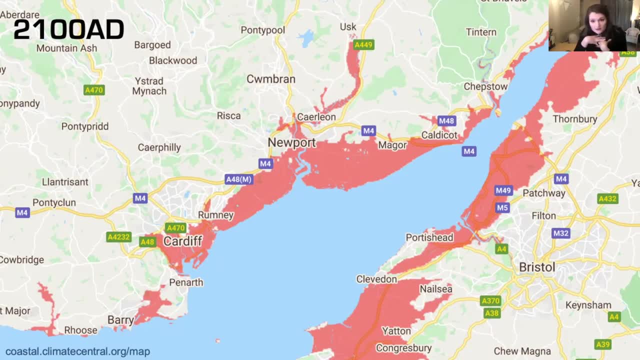 this shows the landscape of my current home in Cardiff and my favourite city of Bristol flooded for children and grandchildren of these cities within only 80 years. so this is 2100, 80 years time, if our atmosphere continues to warm and melt the ice caps at the current rate. 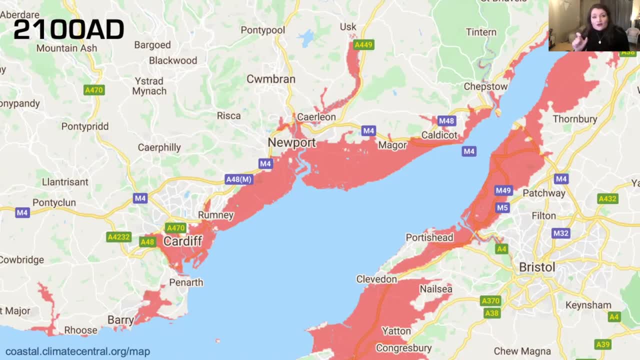 This makes Cardiff the sixth most susceptible city in the world to the impact of climate change, and that's 16 places above London. I'm sure you've all heard the news recently that 2020 was also the hottest year on record. You can actually have a look at your hometown, the website in the corner here. 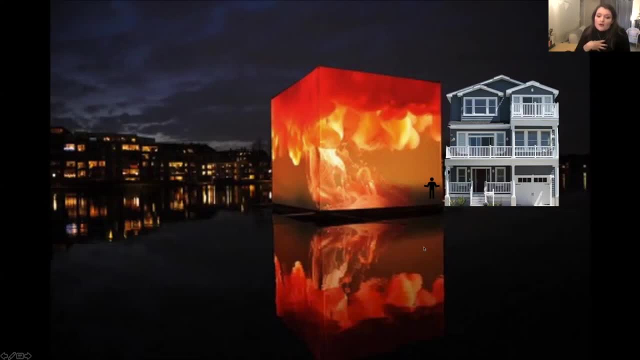 We, the healthcare sector, need to look at our own shortcomings. The NHS is the UK's biggest public greenhouse gas emitter. it's responsible for at least five percent of all UK environmental emissions. The carbon footprint of the UK's greenhouse gas emitter is at least 5% of all UK environmental emissions. 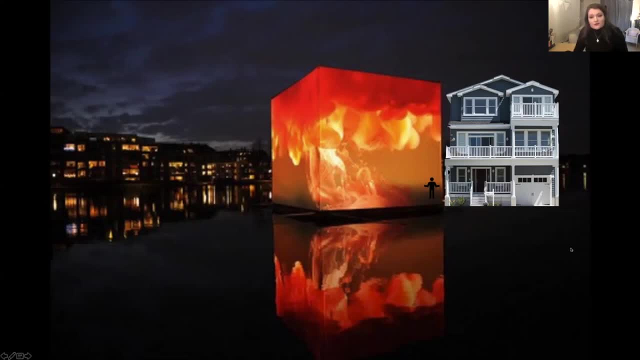 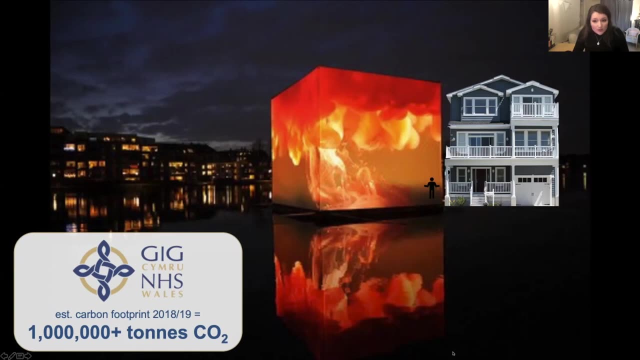 The carbon footprint of the UK's greenhouse gas emitter is at least 5% of all UK environmental emissions. The carbon footprint of the devolved NHS service in Wales for 2018-19 exceeded 1 million tonnes of carbon dioxide emissions, while the latest figure for the whole Department of Health and Social Care 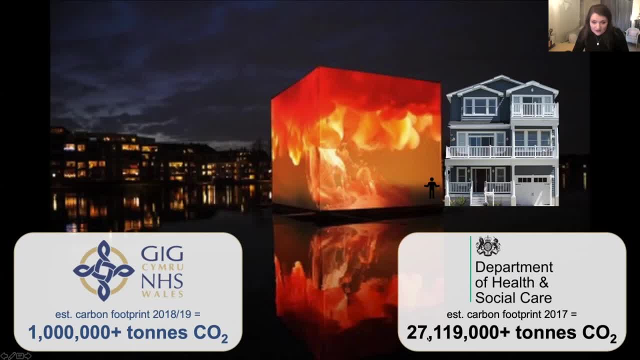 for England exceeded 27 million tonnes. But what does a tonne of carbon dioxide look like? anyway? That's all we ever talk about. This three-storey tall cube in the background represents a tonne of carbon dioxide. in volume, It's equivalent to a three-storey building. You can see the little person I've put in for reference. 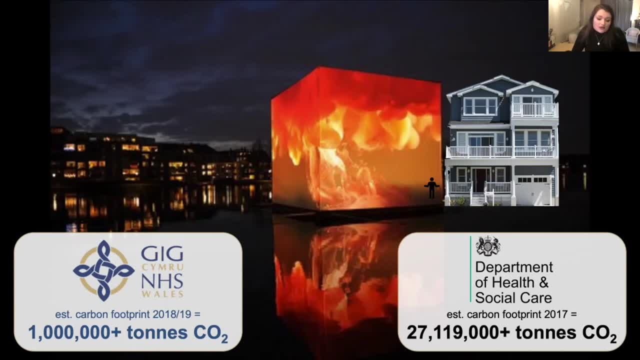 You can see the little person I've put in for reference. We have to imagine the city-sized areas we know and love and live in. they can represent the carbon footprints of our health services. UK health boards are beholden to legislation and policy commitments. 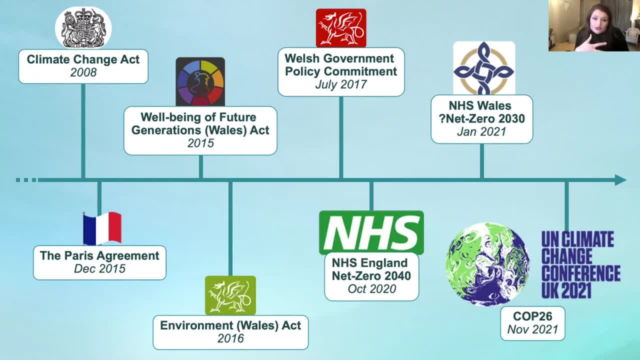 but we can and must use these to our advantage as leverage to affect change. As the name suggests, the Wellbeing of Future Generations Act of Wales here is a powerful tool when considering our descendants and the state of the world we leave to them. I strongly recommend. 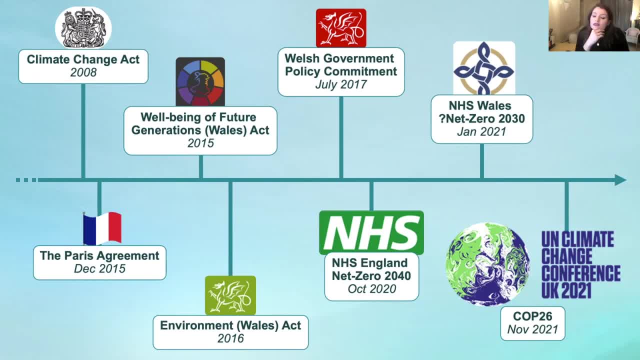 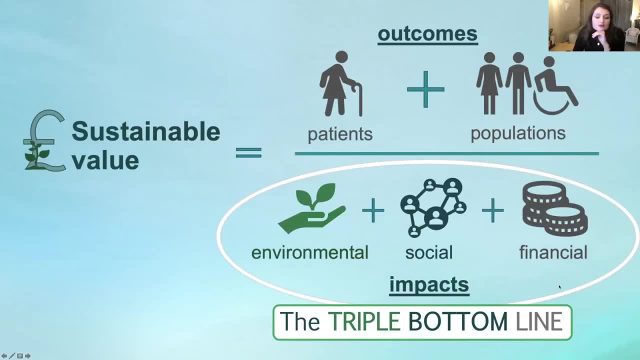 everyone looks it up later, regardless of where you live. it's a fantastic document. okay, what if we continue as we are? what if we don't take this opportunity to do something simple as plugging leaks? firstly, we're not taking care of our staff and our patients- the social value. secondly, we're 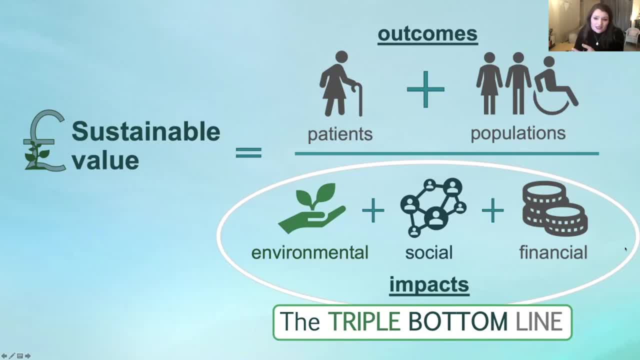 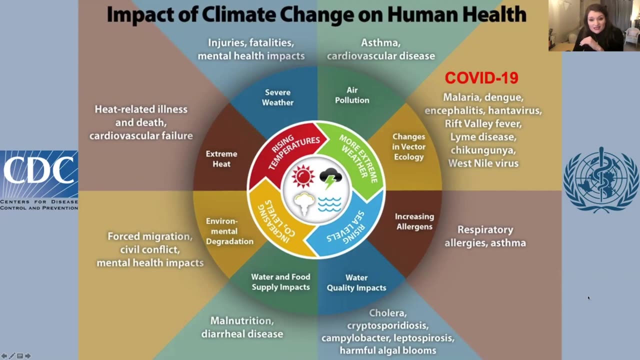 wasting money in an already stretched service. and thirdly, the environment will not forgive us, nor the populations who follow us, and that's known as the triple bottom line. when we consider all these factors in sustainable value, climate change has the potential to undermine the last 50 years. 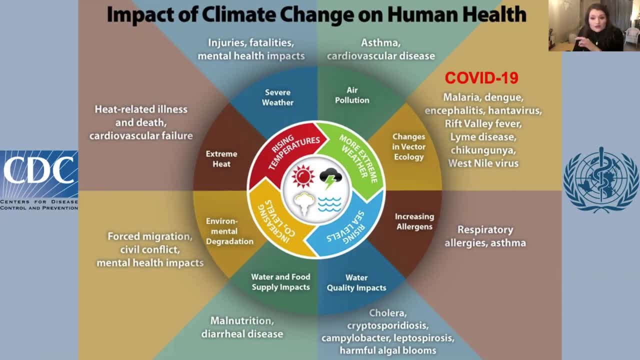 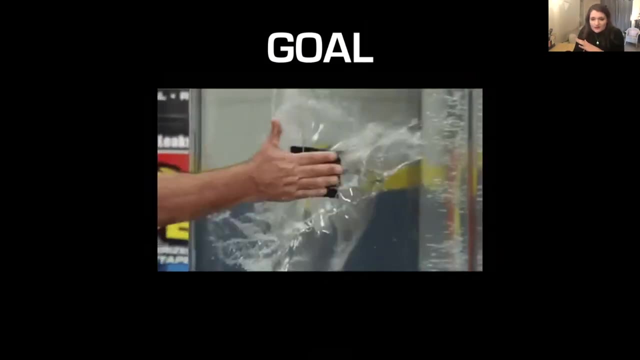 of global gains in public health, the results of which are shown both here in this diagram and evidenced in our current crises and pandemics. they'll simply recur, and likely more often so. our goal for this project is plugging the leaks. this is not about clinical behaviours. 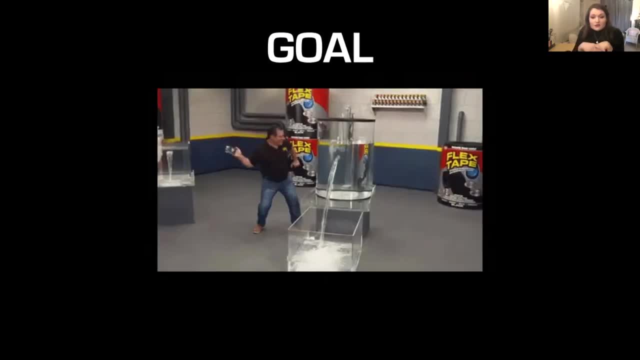 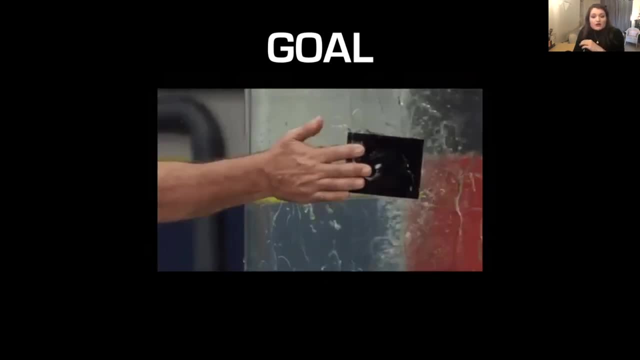 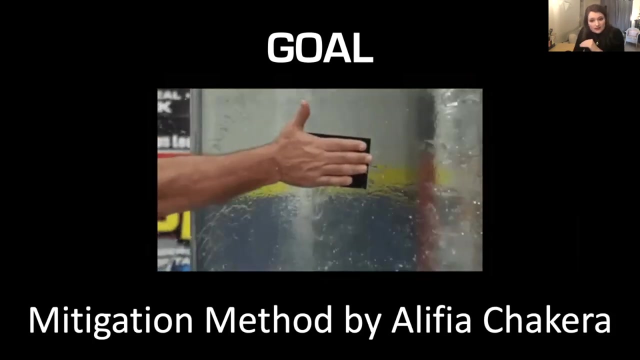 clinical choices and especially is not about denying a vital medicine. we are trying to investigate and mitigate the avoidable problems arising from the ageing infrastructure of a stretched healthcare service. alifia chikara has done just that. her work has succeeded within the theatre and anaesthetics department because she has 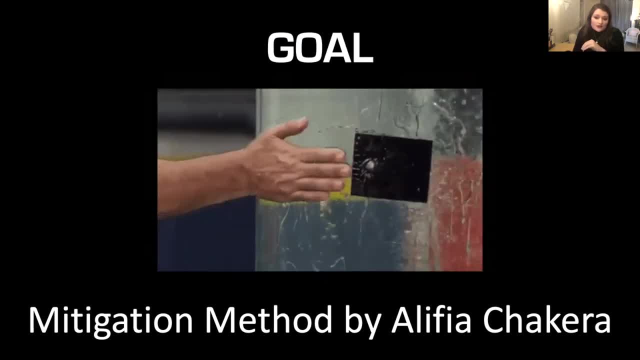 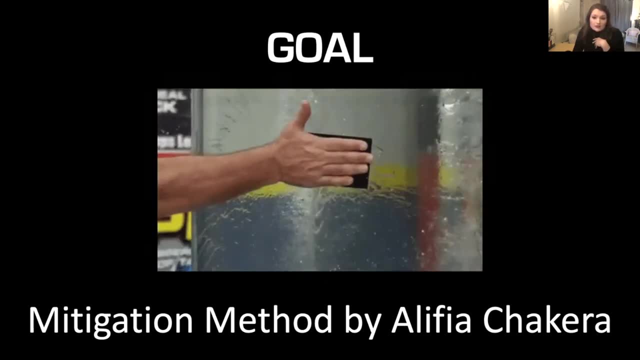 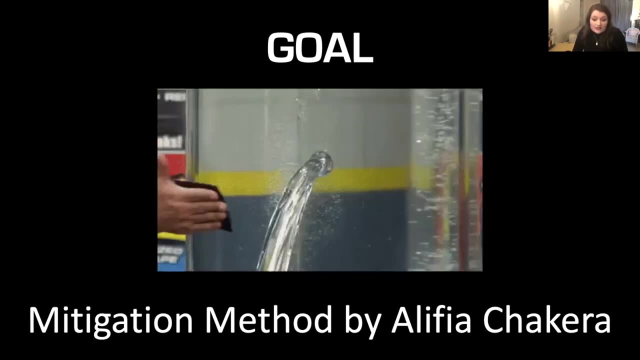 pioneered and developed this method. i challenge all other specialties present at this seminar to consider the method variables within our spheres of operation, whichever background and discipline you come from, because this is new and innovative work, not without troubleshooting updates, and it's very exciting. so, thank you, alifia. i'll stop sharing and hand over the screen to you. 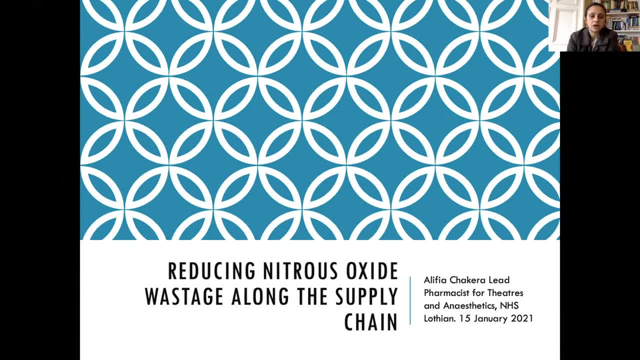 i thank you for taking time out of your busy day to listen to the progress i've made on reducing nitrous oxide emissions within our acute sites. i've spent about 24 months working on this. it's been a real labour of love, so i really do appreciate your time. 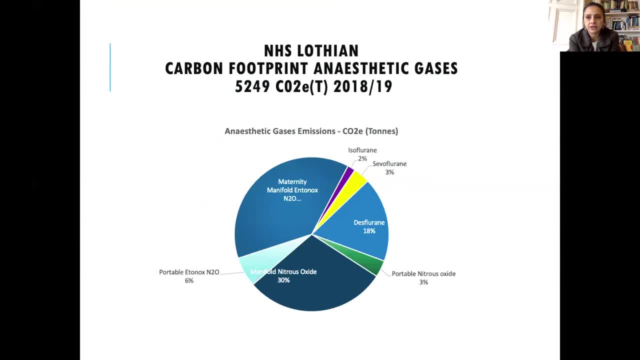 when i first arrived, we hadn't actually done any carbon footprinting of anaesthetic gases, so this slide shows our early attempts, or what the footprint looked like when i first arrived. you can see the volatiles on the right corner. they make about 23 percent of the carbon. 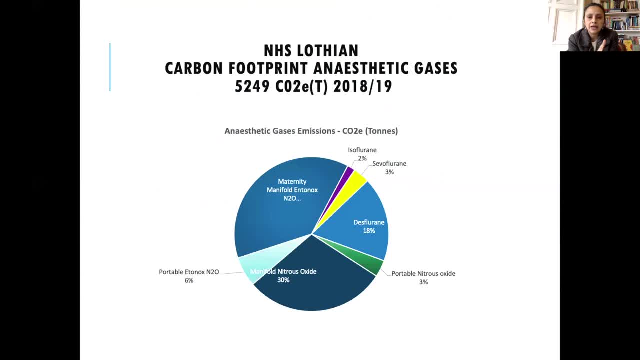 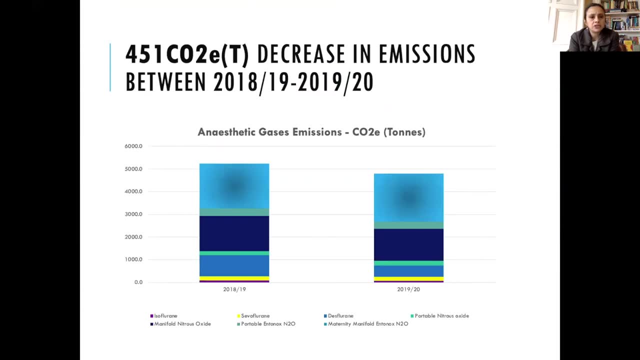 emissions and the rest is made up of nitrous oxide products. now that 23 has more than halved. the following year, which is typical of many health boards, we reduced our emissions by 451 tons. that was chiefly due to reducing desflurane use, but also the rollout of close. 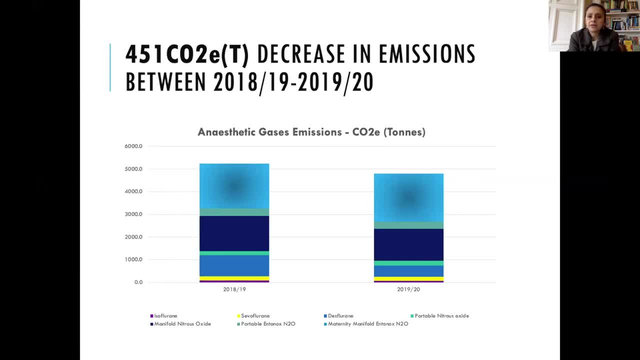 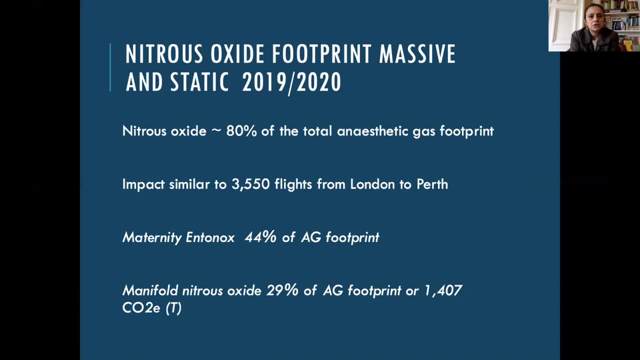 circuit anaesthetic machines also helped. we did not make a single dent, despite education on the nitrous oxide footprint, and that was really concerning. so the nitrous oxide footprint's massive. it's close to 80 percent at the last financial year. for our total footprint its impact is similar to three and a half thousand flights to perth and most of those emissions are 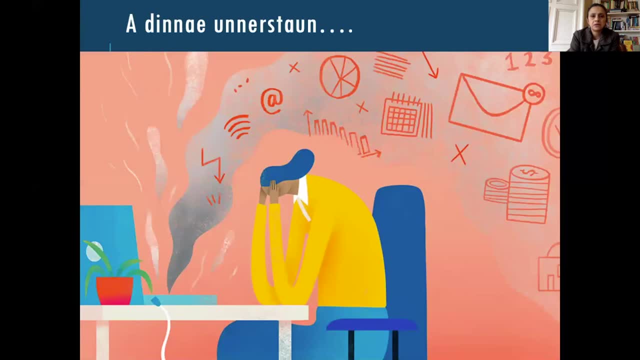 accounted by the antinox and nitrous oxide manifolds. what to do? so we were baffled. we have a really vibrant green anaesthetic machine that's been working for us for over 20 years and we've been working on a number of projects. we've been working on a number of projects we've been working on. 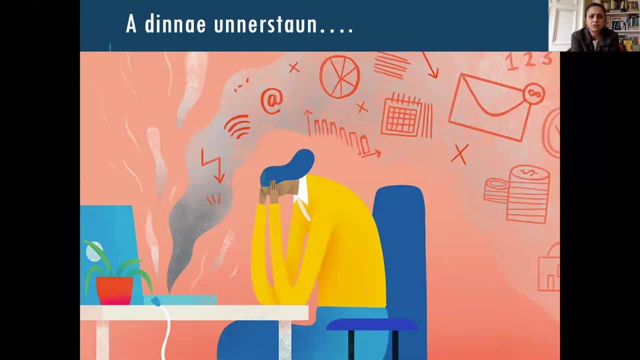 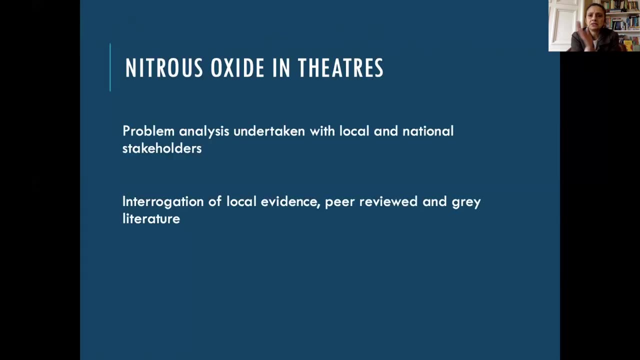 environmental data, tccs. we really have a strong team, but we're really honestly baffled. despite all our efforts, nothing was moving. so what to do? i realized i needed to concentrate on this problem and i narrowed my focus to nitrous oxide in theaters. to be fair, that because i work in. 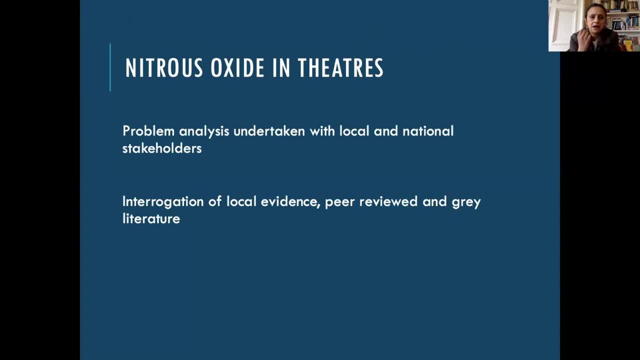 theaters and anesthetic. it made sense in the first instance. i really took a lot of time to really understand the problem and i spoke to everyone, anyone who had some knowledge or interest. i literally wore the carpet out to their door. i just really wanted to get under the problem. 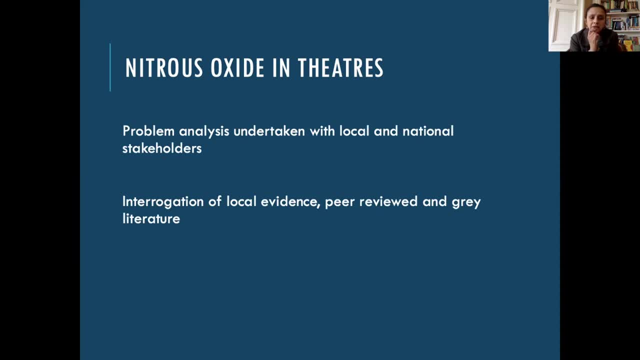 and spoke to international and national, as well as local, stakeholders about this. but also i did a deep review of the evidence and i really challenged and contacted authors about their data and how they may have achieved reductions in nitrous oxide to really unpack what was going on behind the scenes with nitrous oxide and i came to a couple of conclusions. 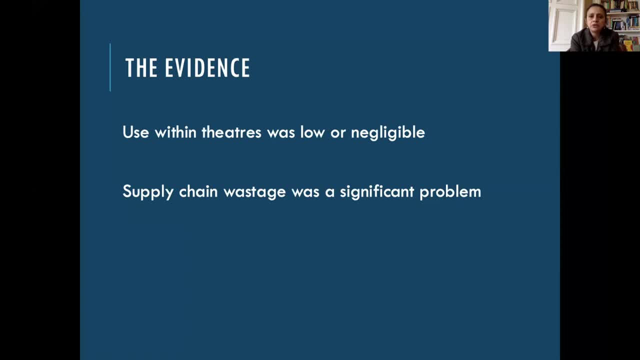 one that, at least in theaters, use was really really low. contemporary use of nitrous oxide had really diminished over the last 30 to 40 years. i believe that supply chain wastage was actually a real problem, so this tipped a lot of the thinking on its head, at least from a clinical 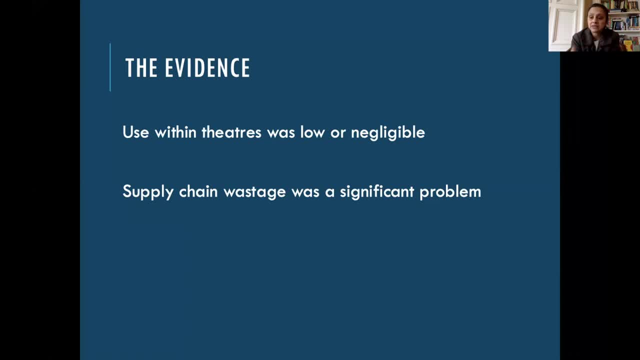 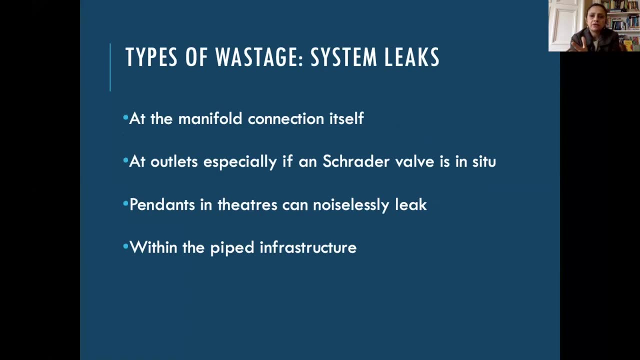 perspective, because nobody had thought of that before. so that was interesting and so i had to set about to prove it. so how do we lose that nitrous oxide? where does it go? so the first area that you'll find it can go is in leaks. the manifold connection itself will leak. so if you don't, 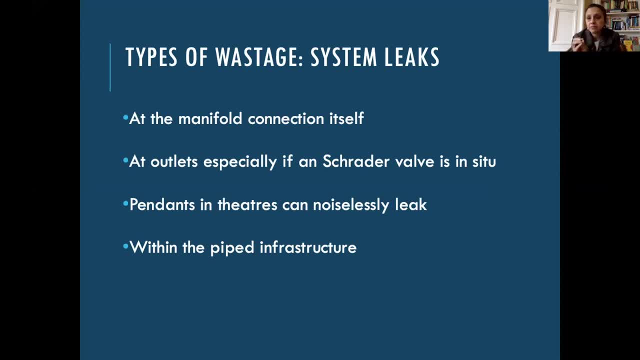 test for leaks at that connection using a soapbox. then you are able to test this leaky connection spray and that bubbles and you'll know there's a leak. that can be a source of a chronic leak. outlets, especially the Schrader valves in situ, are prone to leaks. they're under tension. 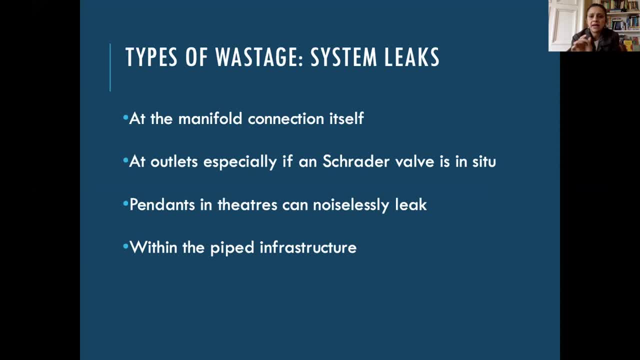 outlets and pendants in theatre can also leak, micro, have micro leaks and they will be really quiet, you won't hear them. but also you can get leaks within the piped infrastructure. now that's a problem too. so if you do get a leak in the private piped infrastructure, that will 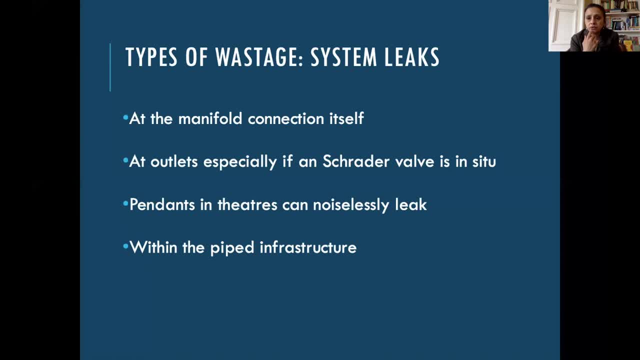 need to be escalated to a senior gas engineer for for a review. now it's really important to understand in all of this: if you have a series of micro leaks amassing, say, one litre a minute, you will lose 43 000 litres a month. translating that up to a year, that's 516 000 litres over the. 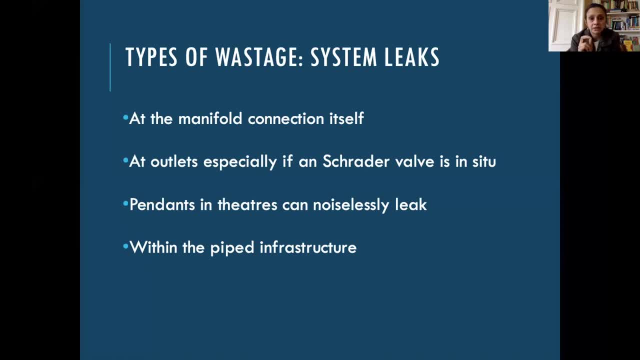 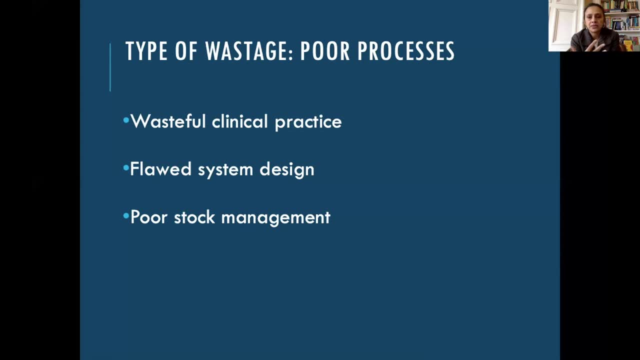 course of a year. that loss is catastrophic in terms of environmental health. our knowledge has moved on and actually we we can't really tolerate those losses anymore. another type of waste is poor processes that can cause a lot of damage to the environment and that can cause a lot of damage to 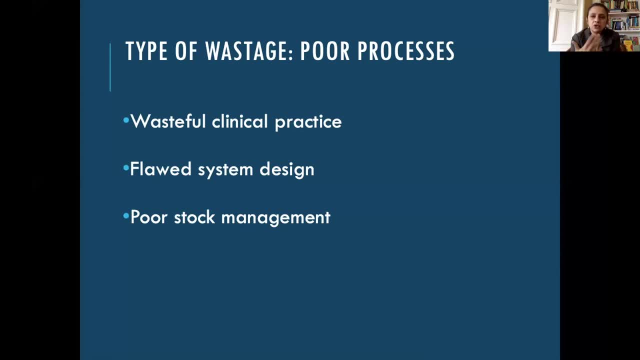 the environment and that can cause a lot of damage to the environment. this is also interesting. when you looked at the evidence, they'll talk about clinical practice and wastage. i believe that's a drop in the ocean, or dribble in the ocean, compared to other losses we can face in. 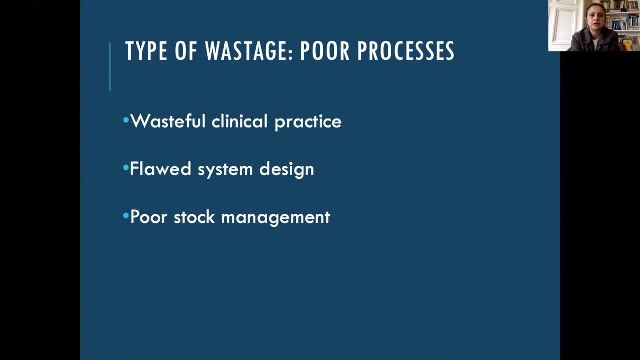 a system, but i think it's really important to focus on really good clinical practice. flawed system design is another thing. you can have old anesthetic machines that don't sort of turn off immediately or you don't hear an alarm bell ringing, or the pressure in a system could be set a bit too high, so that can mean that your cylinders 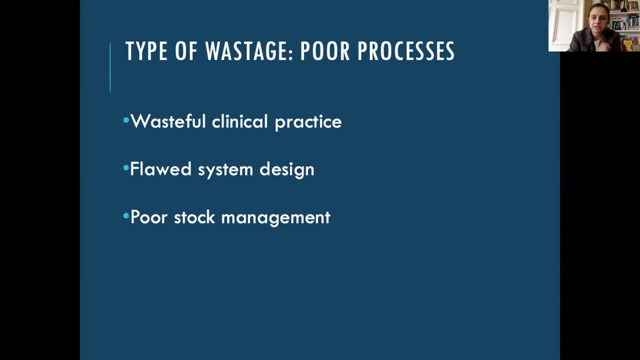 are returned a little bit too early. so there's all those residual um nitrous oxide in a cylinder and that you know, if the pressure is set a bit high that can be a problem. the other issue in this system design is that our specifications for nitrous oxide are set. 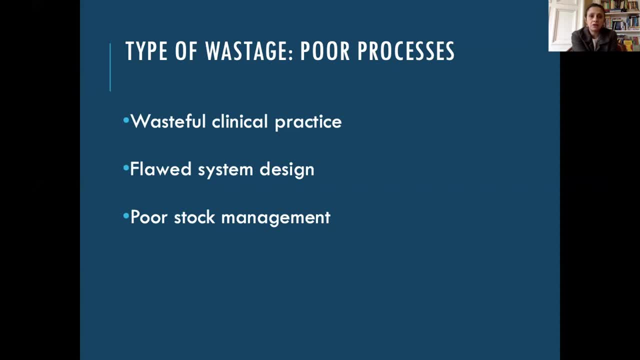 very high, so that creates pressure in the system. so our hospitals, or old hospitals, are designed to deliver very high levels of nitrous oxide compared to what's actually really needed in contemporary practice. the other area is poor stock management. this could come in the form of over provision, stock expires on the bank or just poor stock rotation. 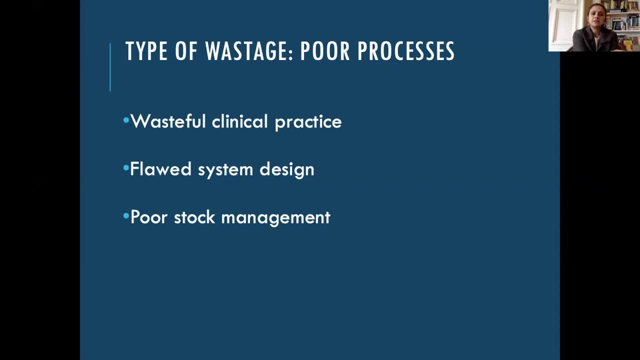 so all of these things need to be thought about. something you need to remember is, as stock goes back to our supplier or our medical gas cylinder suppliers, at the moment, under ec legislation they're obliged to vent that to the atmosphere. in due course that will change. i really hope it will. 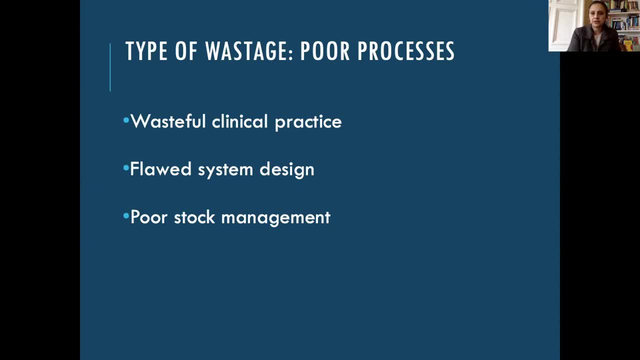 but right now, all that waste is part of our footprint and it's something we need to be really mindful of. another type of waste is theft. now it's really important to keep your cylinders under lock and key. that may seem really up screamingly obvious, but often cylinder security. 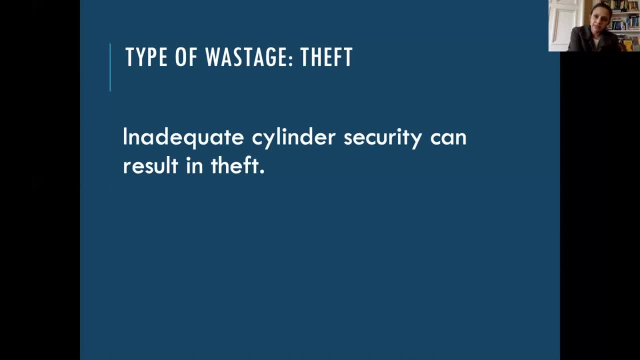 is a problem. so i'd be pretty impressed if a thief managed to wander off with a big bentonox ew cylinder, but you know they could pull up a lorry if, especially if they know a cylinder store is left open. so really keep your cylinders under lock and key, because they do contain a street value. this. 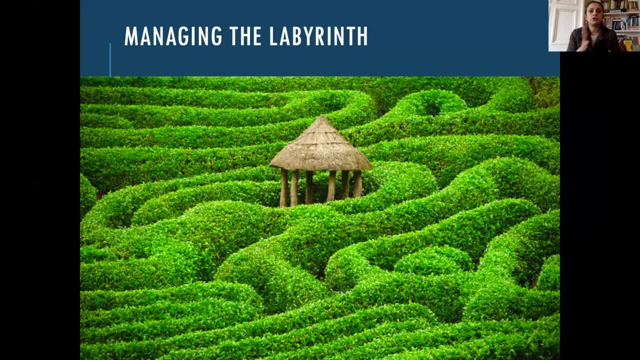 was a really difficult problem. there's a lot of people involved in the supply of nitrous oxide, in the utility of nitrous oxide. how do we get on top of it? so i spent a bit of time thinking about this and looking at the waste management literature and i decided on utilizing a six, a lean six sigma. 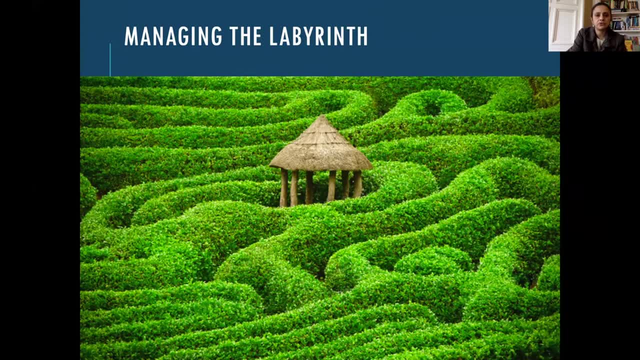 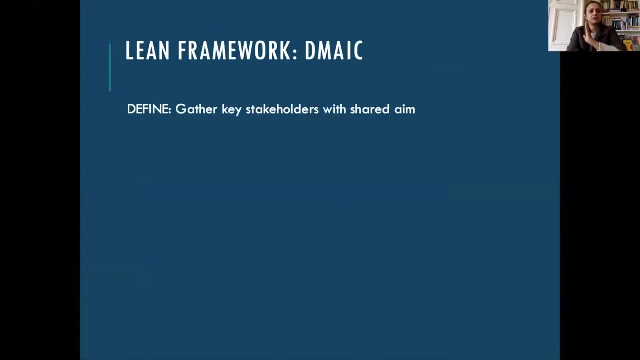 structure, which which really helped me a lot and, to be fair, it's something i've used before. so the leading framework i lent on was called dmacc and it was really helpful. so it's a five-step cycle, but the first step you want to do is you want to gather your stakeholders and you want to 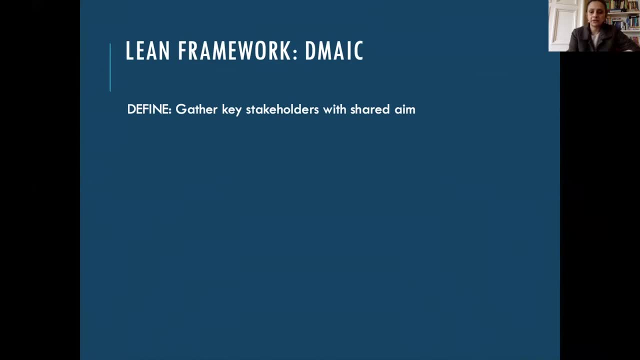 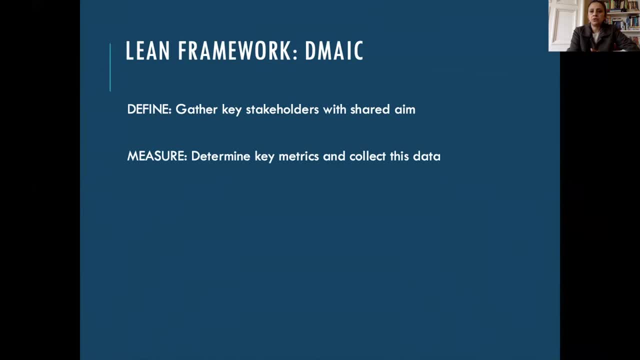 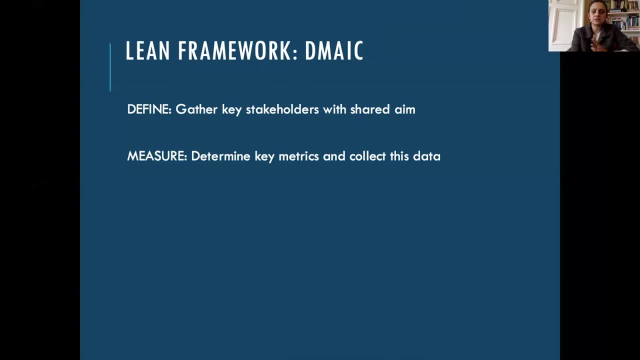 about to do what i was trying to do, or i about to do what i was trying to do, or i couldn't find any information of somebody. couldn't find any information of somebody. couldn't find any information of somebody who's trying to. you know, work on this. 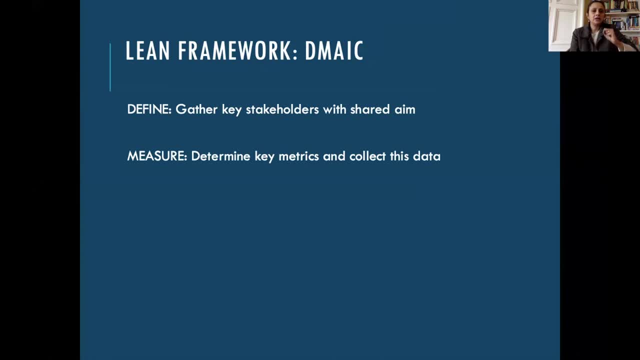 who's trying to you know work on this? who's trying to you know work on this? this sort of level of metric. so i had to this sort of level of metric, so i had to this sort of level of metric. so i had to really decide what my metrics were again. 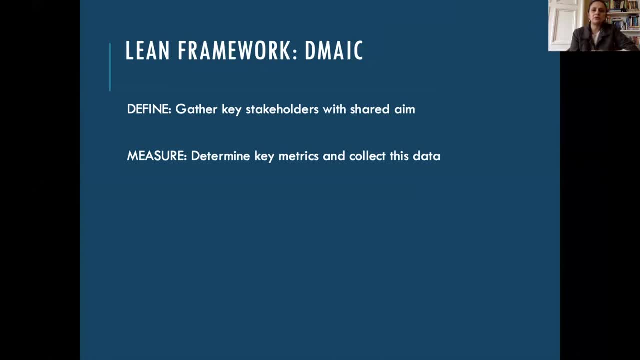 really decide what my metrics were again. really decide what my metrics were again. working with your stakeholders is really important to sort of determine what they are, but also who will set about to collector and how collect that data and how would you pull together that data as well. so this is where the stakeholder 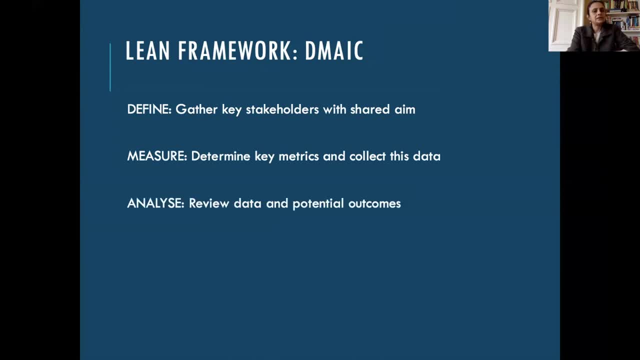 is really important. um, you want to analyze this data. i used a format called decision tree analysis, which allows you to pull threads of evidence out and put them against certain actions, so you can- you can- create a really good map that way. i found that really useful. you should use whatever. 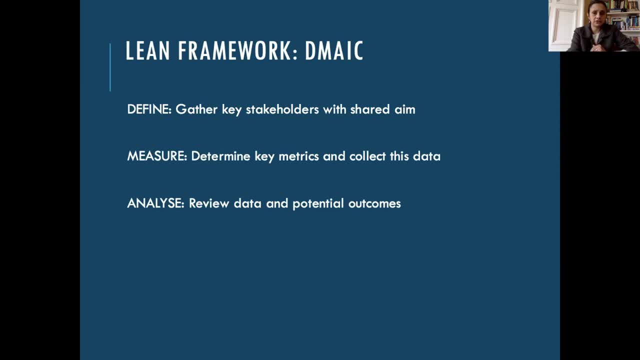 analysis tool you prefer, but honestly decide that as a team. if you are planning to do that now, the next step is to improve, to act on it now. some things are really simple. so if you know that a leak is caused because of a leak at the manifold, that's a pretty easy fix. you introduce, um, you know. 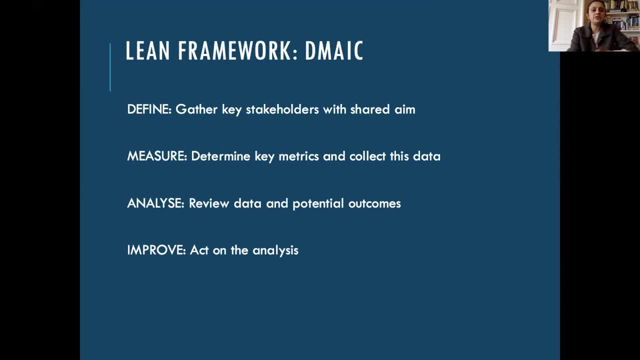 management around that and you know, deal with that problem. but you may find that you need to either decommission a manifold or close part of a service down and that will need escalating and you will need to escalate it and you will need to escalate it and you will need to escalate it and you will 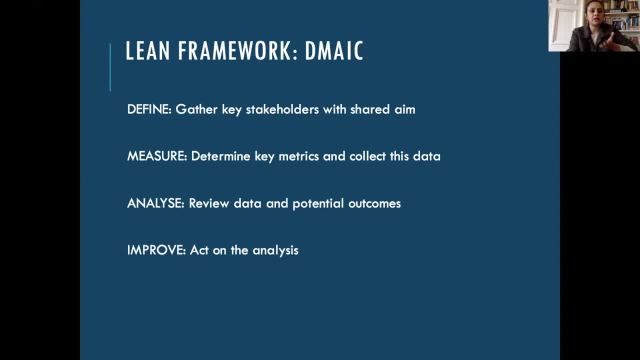 and people like QAS pharmacists will need to get involved. Your clinical leads will need to get involved. So just be aware of that. You will need to. action will also require escalation at times. Control you may discover as you go through the process. 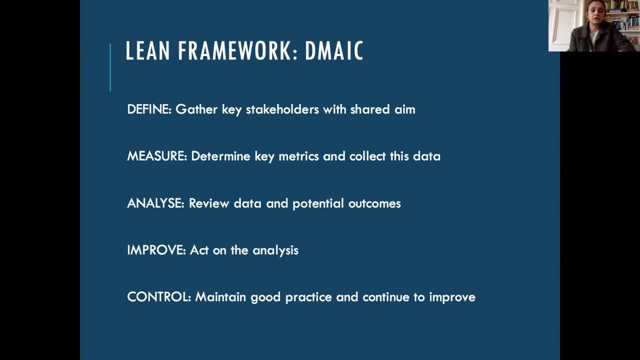 well one. you want to maintain the practice, So you introduce methods of work that are more sustainable. but also you may need to do a deeper review And at one site we've started doing process map sessions- a little bit delayed because of COVID. 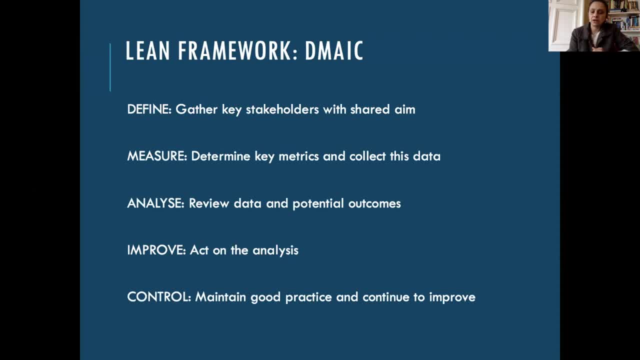 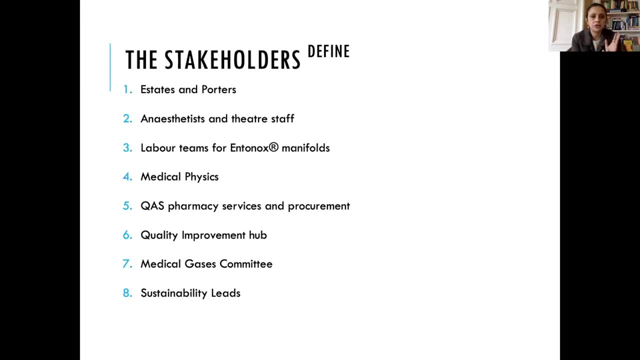 but actually that's already led to some improved practice, which I'm delighted with. So, stakeholders: I put a list of stakeholders here. All of these people are important. You will want to speak to your pharmacy services. You will need to speak to estates and porters. 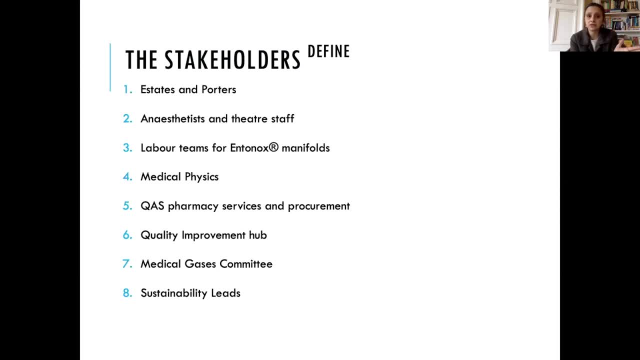 Depending on the project. if you're just going to focus on your nitrous oxide, you will need to speak to the anaesthetic and theatre teams. If you're going to focus on Entonox, you'll need to focus on labour teams. 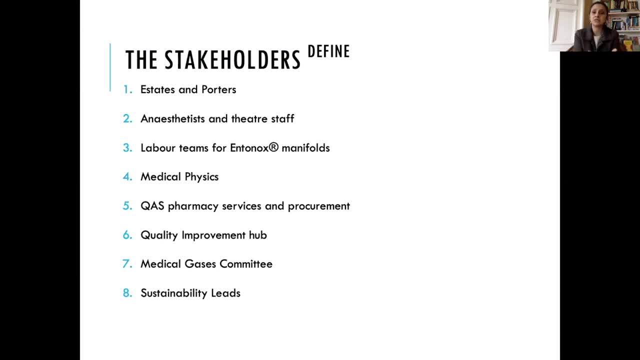 Perhaps you'll want to do the whole shebang. It doesn't matter, But the point is, at some point you will need to speak to the hospital. you will need to speak to all of these people. The sooner you do it, the better. 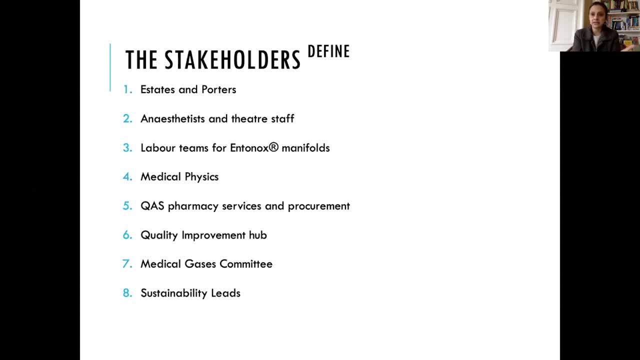 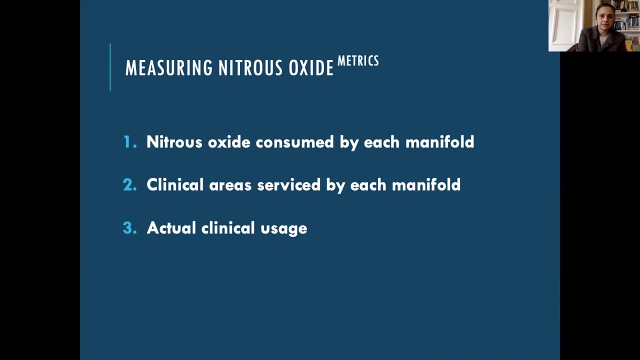 Honestly. if you can speak to everybody and let them know what you're doing and what you're intending, and build real friendships with this network, you will develop a far richer and powerful impactful project. So, measuring nitrous oxide: I worked out those three metrics I really needed. 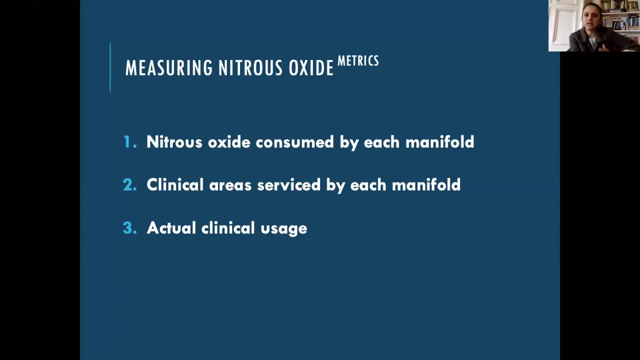 One was I needed to understand how much nitrous oxide was actually utilised by each manifold. This is really important because you can have more than one manifold at an acute site, So you want to know the division between the two manifolds. The next: I wanted to understand which clinical areas 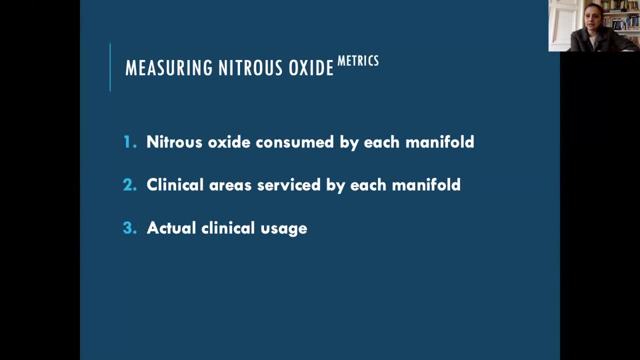 were serviced by each manifold. And finally, I wanted to understand actual clinical usage. What was the actual clinical usage? Okay, so that's important. Now the manifold audit. So it was a little bit like walking on the moon, but let me tell you how to do it. 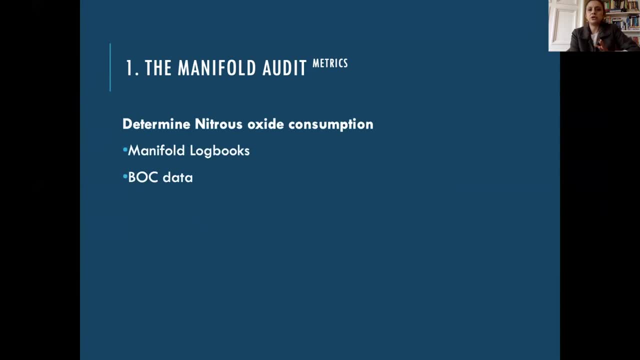 This is great. So the first thing you want to do is: you want, because you want- to determine nitrous oxide consumption. you need to look at your manifold log books- That will help you Understand the volume consumed- And you want to look at this compared to BOC data. 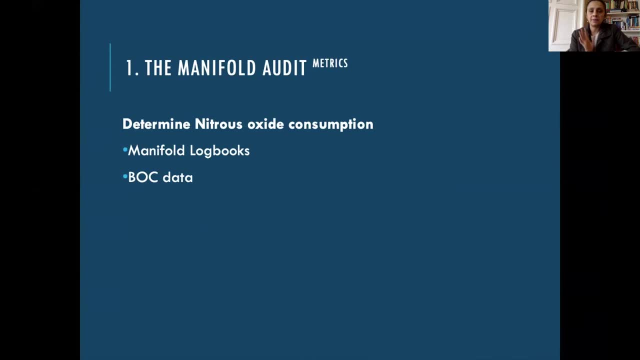 For those of you who don't know who BOC is, BOC is a medical gas cylinder supplier. They supply most of the UK. They supply all of Scotland, I believe all of Wales, and have the bulk of the English markets as well. 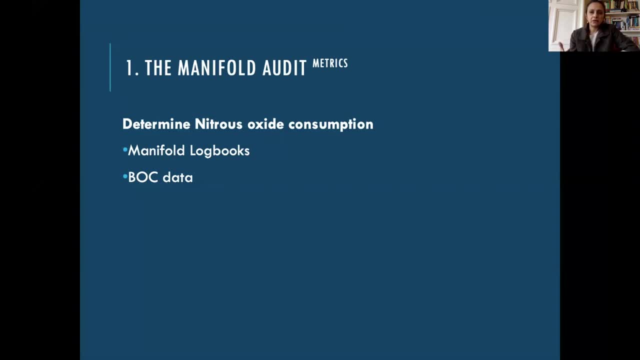 And I think Northern Ireland as well. Now the other is Air Liquide. We don't really use that. We don't use that in Scotland. They follow a similar model. Now the next thing is that you want to also review your manifold management. 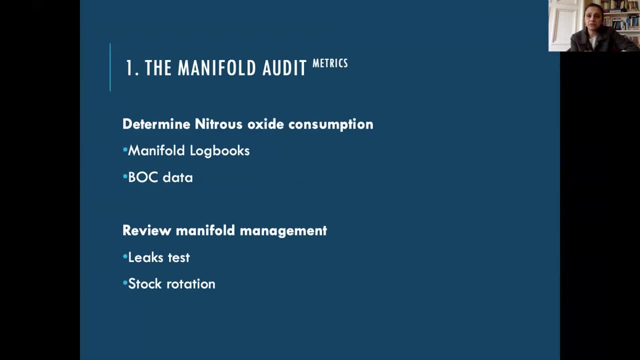 So you want to check that leak tests are being performed. There should be again a log book there. There may not be, or they may. they say, oh yeah, we might do that at the bank change. but ideally a good leak test would be done weekly. 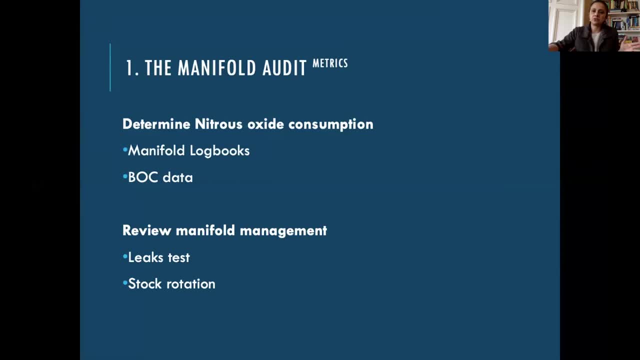 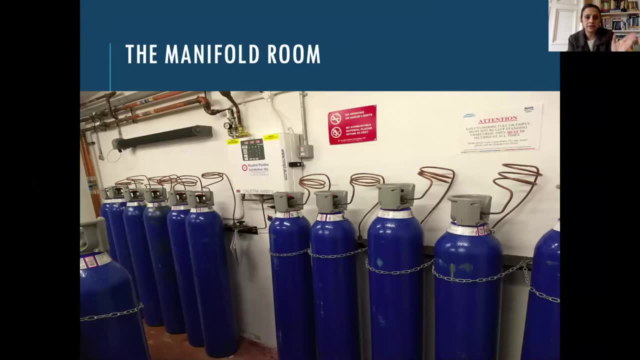 And you want to check if there's adequate stock rotation, And I'll explain this a bit more. So this is a standard manifold room. This is the manifold at the RIE. It's a really big manifold. It's a- it's what they call the six by six arrangement. 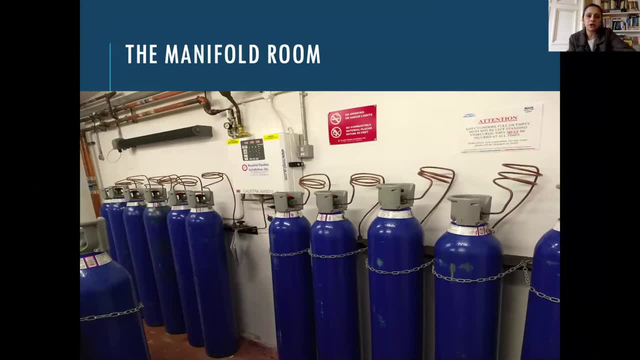 It has six Js and six Js Okay. Now how this works is you'll have say: pretend for a second that the left-hand side is active. When that depletes and the pressure drops in the system, it'll automatically flip over to the right bank. 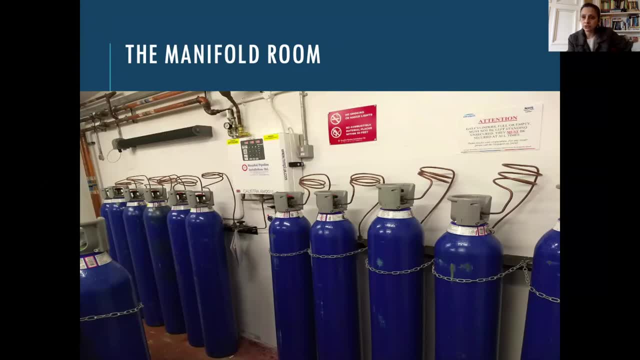 At that point an alarm is triggered to security, security alert porters, portering service, and they will come along within 48 hours to change a bank. Okay, Now, within this there's also- you can't see it in this picture- There's also a small emergency reserve, which I think is completely superfluous. There's no need for it, but there it is, And the only reason you'd end up going to that is if you have a major leak. So now you know these are J size cylinders. 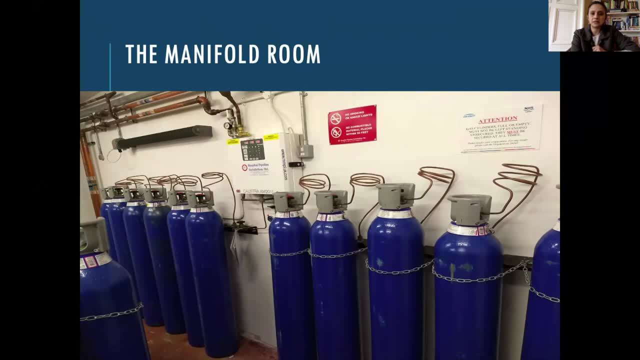 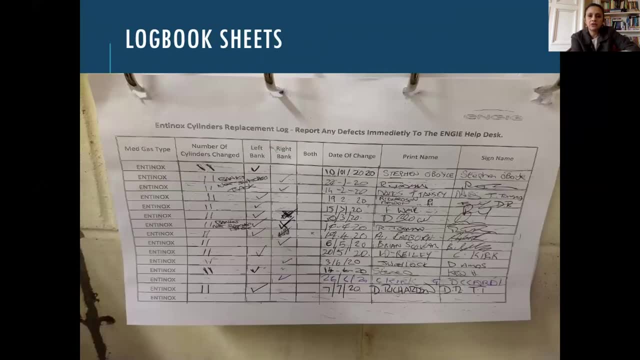 They're enormous. They hold 18,000, 18,000 liters. I mean, the gas is compressed, obviously, but yeah, So they're quite big. This is a an example of a log sheet, Again from the Royal, from their Entonox manifold. 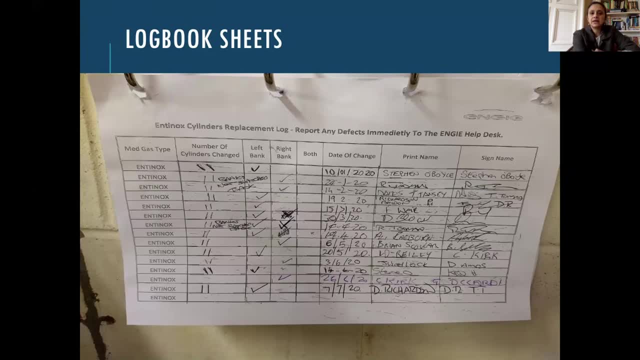 Entonox spelled slightly incorrectly but that's okay. This again just shows you when they, which bank they change, how often they, the date they changed it And from that you can really calculate volume of Entonox, which is the end of that manifold. 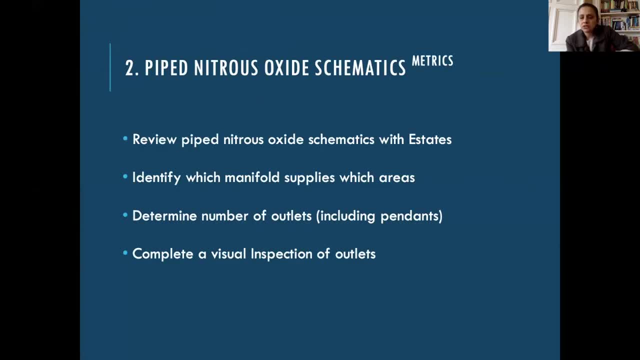 Very straightforward really. Now, the next thing you want to do is look at just schematics. You want to understand which parts of the hospital are being fed by which manifold. Now, to do this, you'll need to speak to your estates teams. 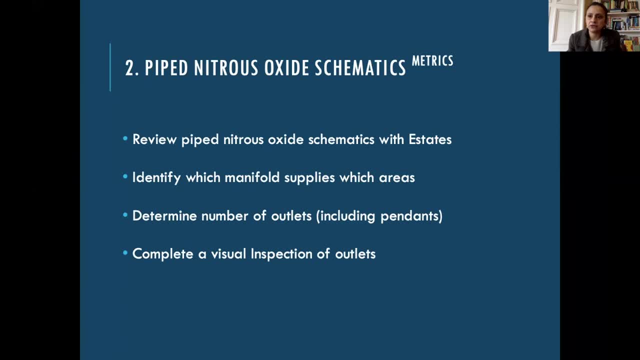 And this is a really great job for the clinical teams to do. So if you're a midwife who's interested in Entonox waste reduction you it's a really fun job to actually go around with the with the estate team. 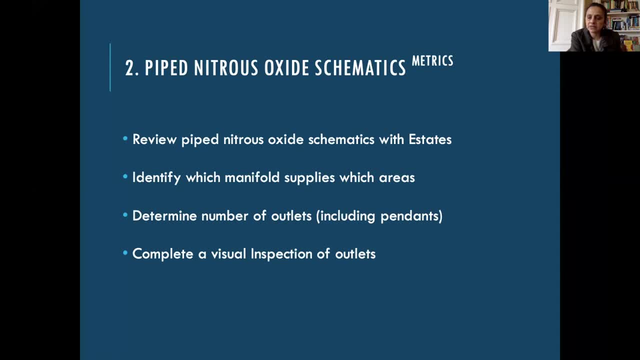 and having a look at the schematics. I know I've looked at all three sites and clinicians actually really enjoyed going out and seeing those schematics. The other thing you want to do with all of that is that you want to also complete a visual inspection. 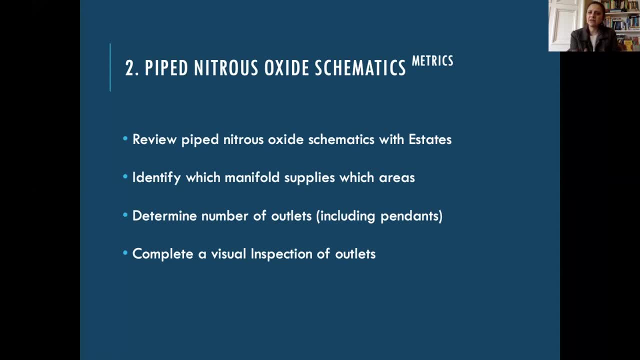 of those things just to make sure the schematics- and they can sometimes be a mismatch, especially if some work's been done that's not being documented properly. So just a sense check by doing a visual inspection is really, really useful. From that you want to determine how many outlets. 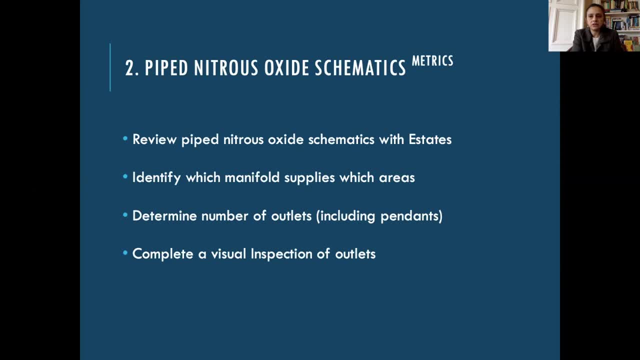 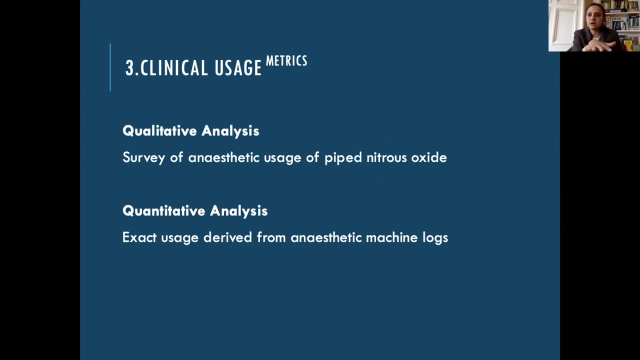 and pendants you have. So I think that's really really, really helpful. So make sure you do do that. The next thing in all of this is your analysis. Now I've put qualitative and quantitative analysis here, And I think both are really, really important. 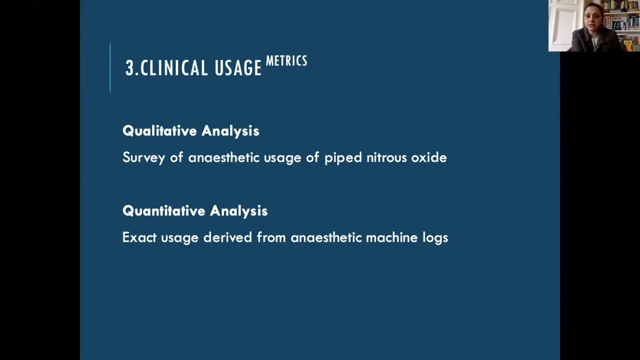 because, for example, when we started the project at the first site we were in early pandemic mode, So surgical activity completed had depleted. If we relied on quantitative analysis from you know, taking it from the anesthetic logs, we would have been in trouble. 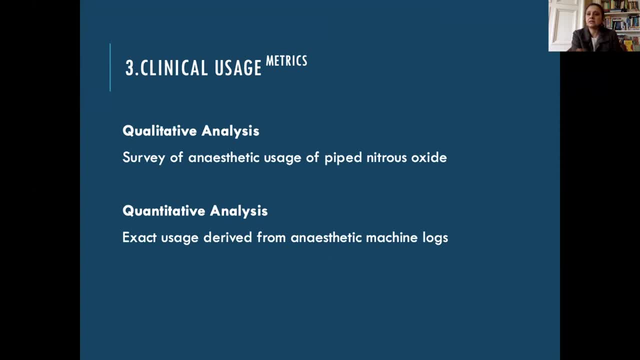 because it would have given a completely false picture. Qualitative analysis gives you a sense of previous use, but also projected use, So I think it's really really useful to look at both and compare those two sets of data, if you can get it. 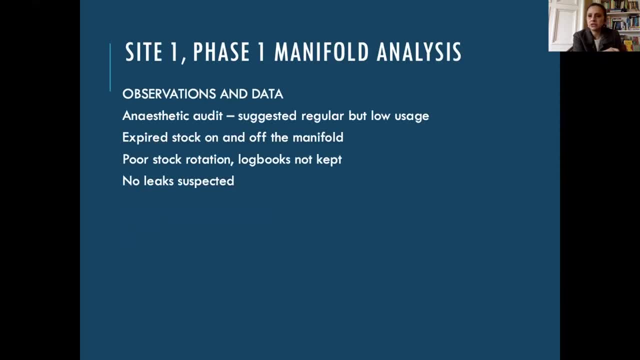 The site one phase one manifold analysis. the anesthetic audit suggested low but regular usage. So that was important. But on this manifold stock was expiring, on and off the manifold It was. I mean, it was a disaster. There was really poor stock rotation. 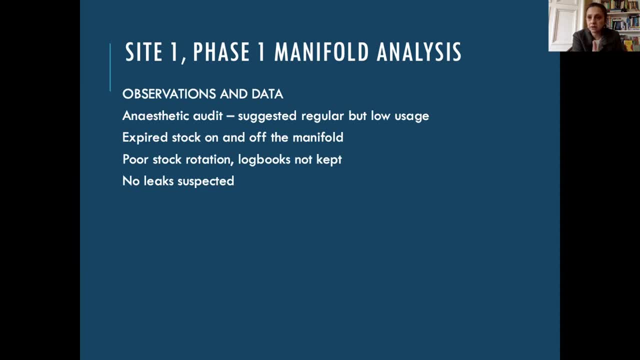 Logbooks weren't kept. However, no leaks were suspected, So that was great. So actually, the banks of cylinders were just going out of date, So the waste was due to over-provision. That was essentially what was happening. We took a decision to reduce the supply of nitrous oxide. 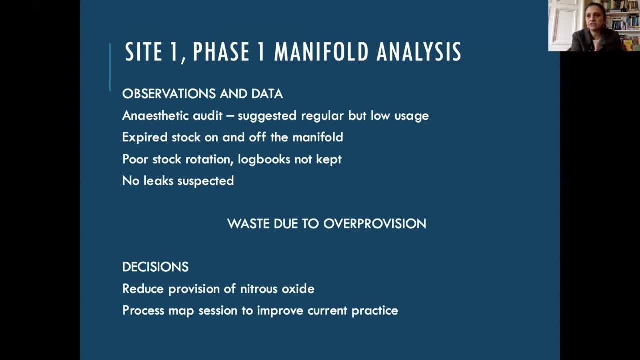 but the anesthetists have a long-term goal of maybe sort of removing that manifold altogether. but they're working towards that as a team. So we've gone from a four by four arrangement to a one by one arrangement And that seems to be okay at the moment. 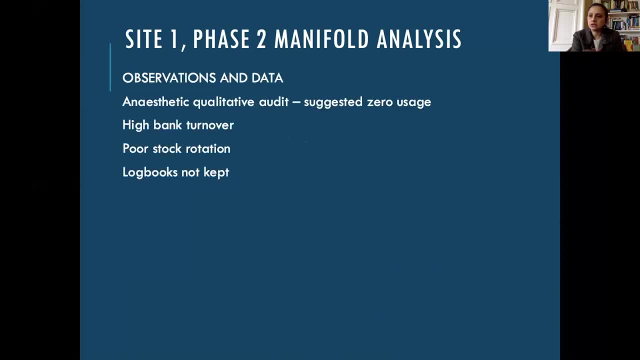 The next one was the same site, but the secondary manifold. The quality of order was interesting. It suggested zero usage, but there's a really high bank turnover. Within a 10 month period, we'd exhausted 88 cylinders And in fact this is what highlighted the problem. 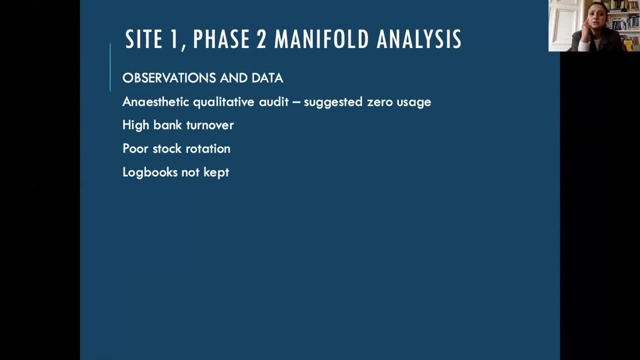 for me to go to this site first because it honestly did not make any sense. There was again terrible stock rotation, The emergency bank was just expiring, They weren't integrating into the main banks and logbooks weren't kept. All of these things did not bode well. 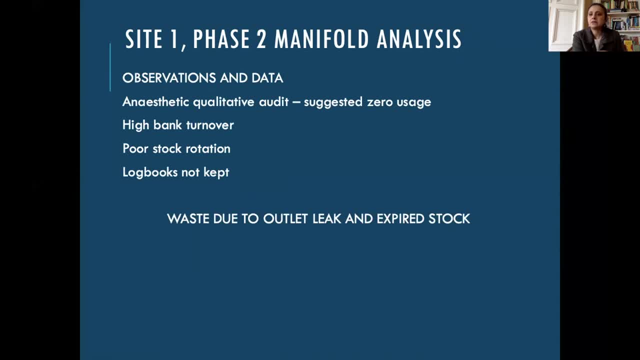 The waste there was determined to be from an outlet leak and, to a lesser extent, expired stock, So the decision was taken at the back end of 2019 to terminate the leak. Later the team took the decision to decommission a manifold And I think that was completely pertinent. 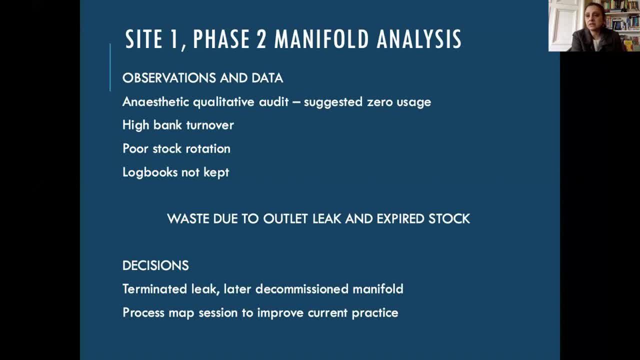 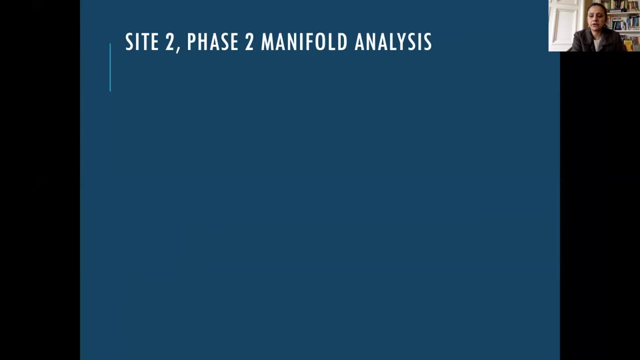 completely reasonable choice. This site needed. this is the site that needed deep review. It still needs review of its management of medical gases And, like I said, process mapping is a great way to bring the team together to have those discussions. So site two completely different scenario. 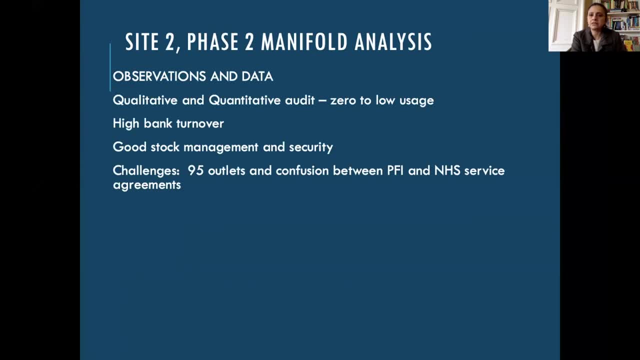 The main thing here was we looked at both qualitative and quantitative analysis. It's a bigger site covering 15 theaters as well as an ED department. There was very low usage, determined by both bits of evidence, but there was a really high bank turnover. 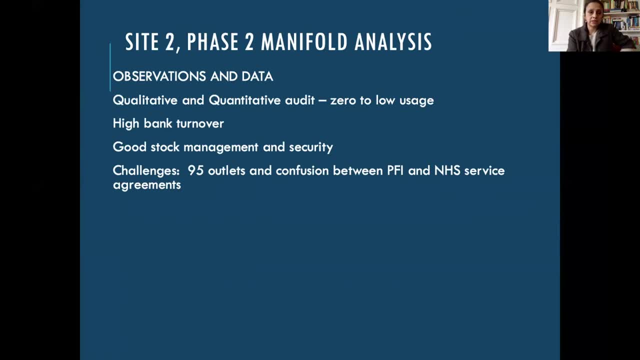 excellent manifold management, really good security. The challenges we had was there were 95 outlets. We're talking about kilometers of pipe work and also confusion between the PFI and NHS service agreements. So that can sometimes mean that your service arrangements can fall down very, you know, very- badly. 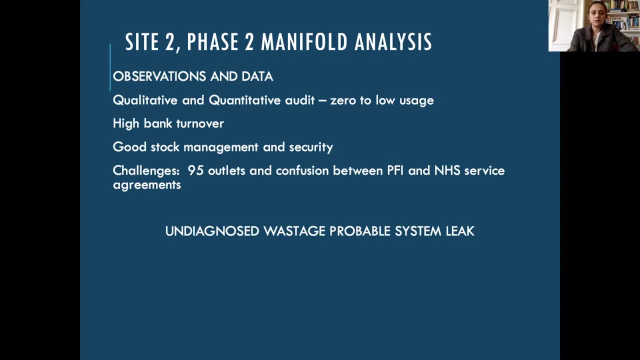 There's a high nose wastage problem there, most likely due to a leak. The decision has been taken to decommission that manifold. We're working up to it. We're first providing some leaner supplies to low usage areas, but then the plan is to decommission that manifold. 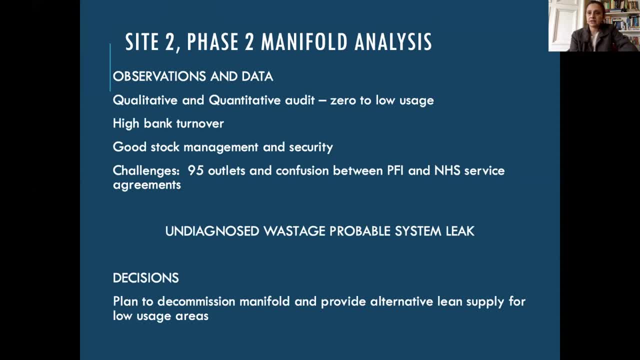 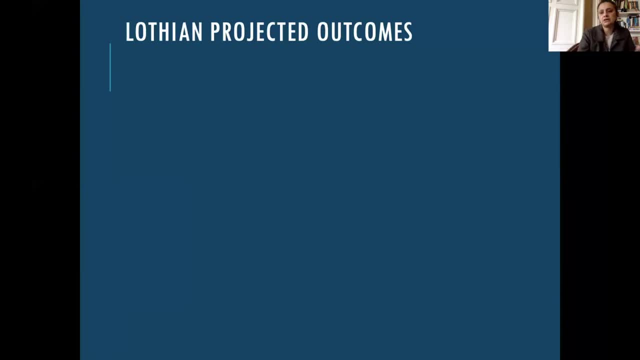 because it's clearly just been over-provided and over-specified for that site. Now Lothian projected outcomes. So what does that mean for Lothian? What have we achieved? It means the projected for site number one. we look like we'll probably reduce eventually. 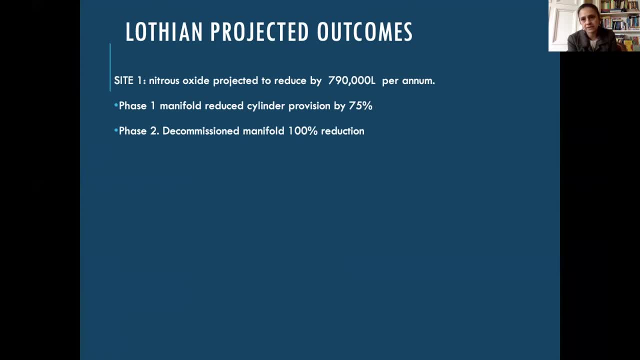 790,000 meters per year, which is great, which is really, really good, And takes that site into a more realistic, you know realm of what nitrous oxide use would look like. The second site will, from that phase two, manifold. 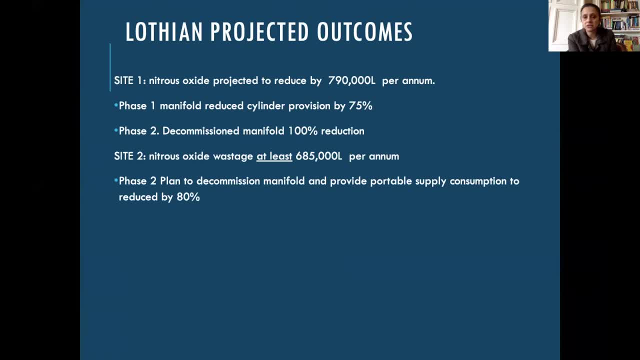 we'll lose probably 685,000 meters with our mitigation measures And that will translate to 850 carbon equivalents in tonnage of emissions lost, which is great. So that's similar to about 700 flights to Australia, So I'm pretty happy. 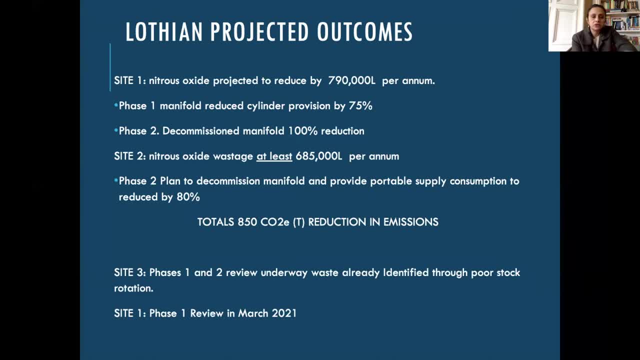 So we're still continuing our review. Site three: we've looked at phase one and phase two and we've already identified waste through to bad stock, to poor stock, rotation and over-provision. Site one: phase one, that the midwives and the obstetric teams have got in touch. 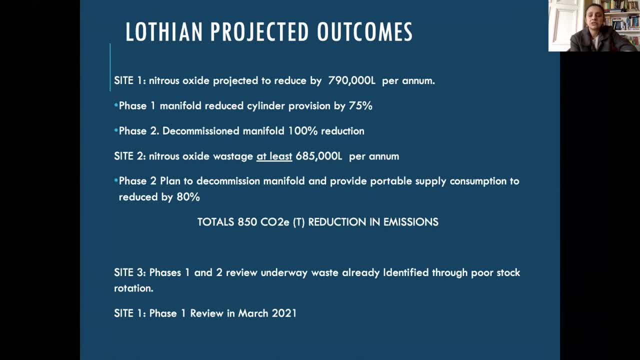 and they would like their Entonox manifold looked at, which is wonderful. Plus, we're planning to look at the manifold- the nitrous oxide manifold- there too, which we already suspect, just based on common sense, that it's probably leaking. So is Lothian an outlier. 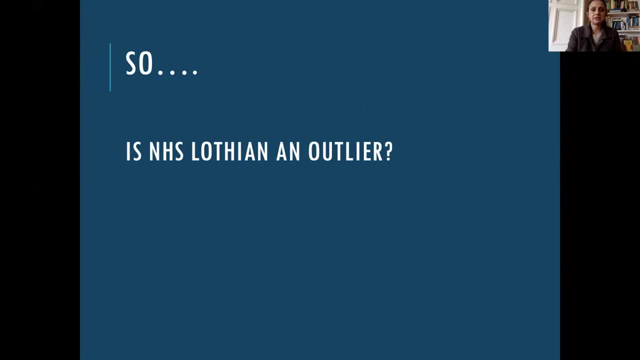 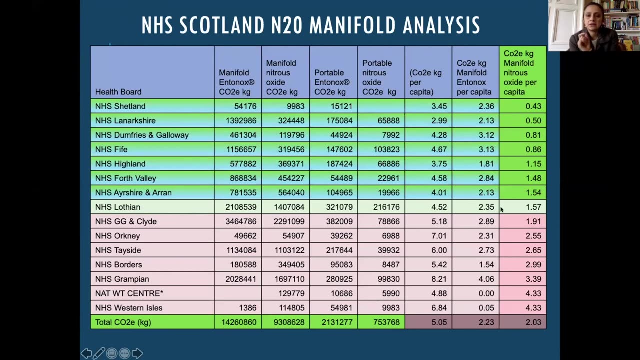 Is it a bit of an oddity? Is it just leaky? Well, the answer to that is simple: no. If you look into the yellow lane on the right-hand side, that indicates that actually Lothian's emissions per capita, based on its healthful data, is on the median. 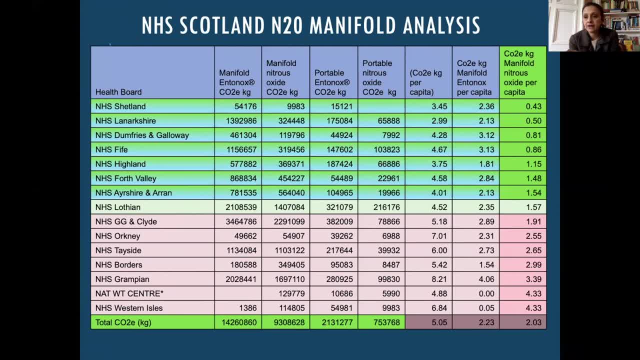 Now I mean this is a very coarse analysis, but it's well, it's below the average. It suggests at least half, if not more, of our health boards. the manifolds are leaking. I think leaks are a really core part of the problem now. 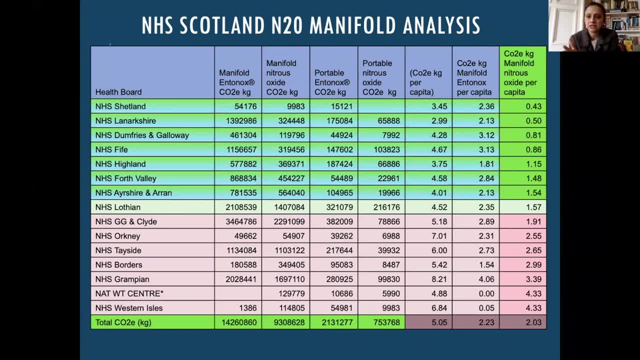 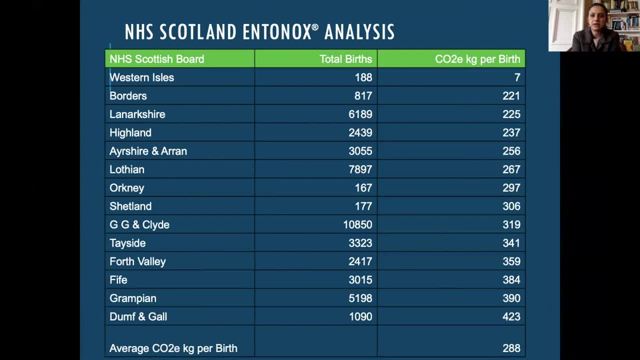 And knowing what we know now about nitrous oxide, we can't really tolerate. Now what does that mean for Entonox? Is Entonox a problem? I think it is. I think it is a problem If we look at the right-hand side here. 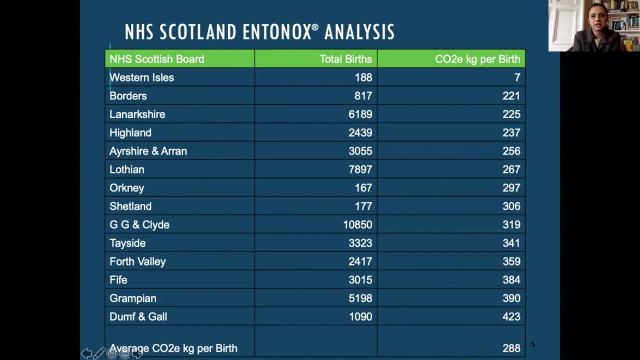 you can see the average is 288 CO2 equivalents per kilo per birth for NHS Scotland. Now Lothian's below below 98% that. but we can see that other health boards are consuming a lot more. that does suggest a leak and 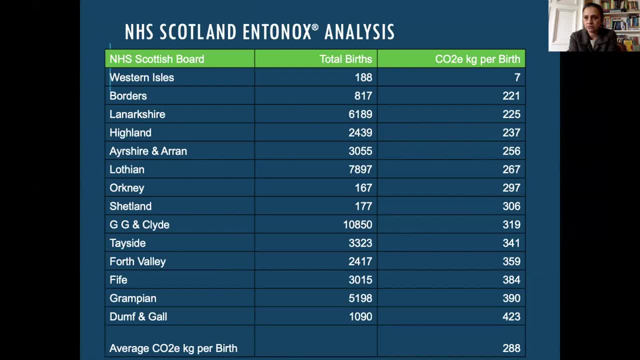 we're already suspicious that we have a leak um from our royal infirmary- a big amount of antinox manifold at the royal infirmary. so this is interesting and honestly i will keep you posted. but i do think antinox manifold- leaks from antinox manifolds- are a problem. there is one hospital down. 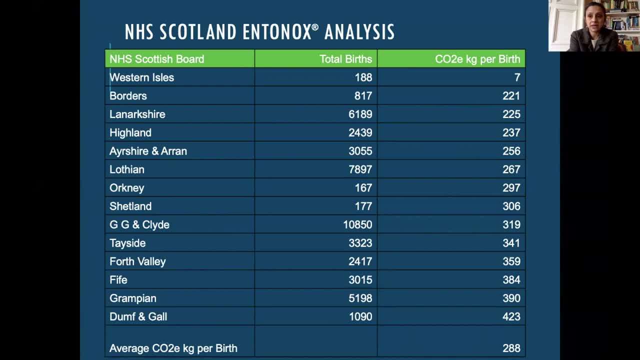 south who's been in touch, and they're roughly averaging 900 kilos in carbon equivalents per birth. uh, there is something seriously wrong. i mean that's just not. that's just not. that can't be real. you kill your mother with that amount. it's not going anywhere near a mum, it's, it's. 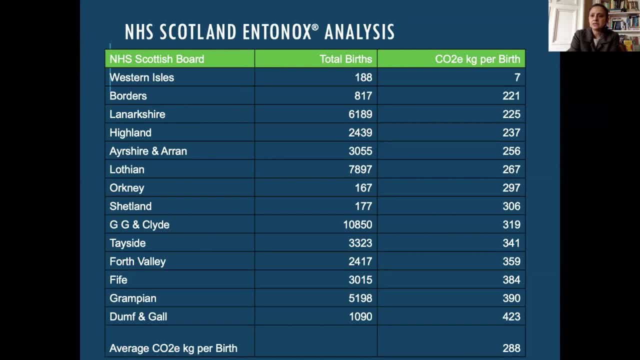 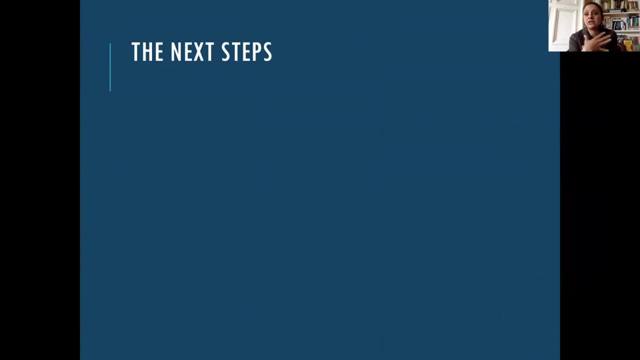 it's leaking before it gets, gets into her. now these things are all important. um, the other thing is the next steps, and before i move on to this slide, i know that i know i'm very interested in technology and green technology to capture a lot of these emissions. but before we even look at 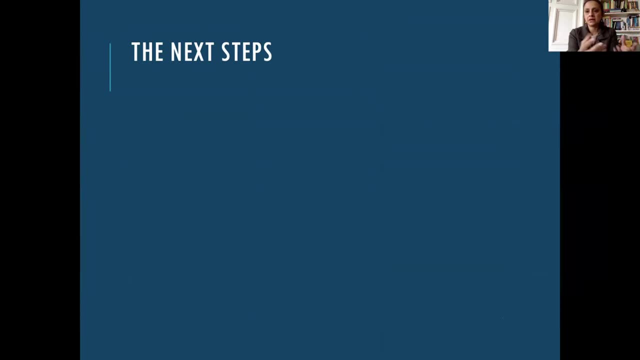 catalytic cracking technology which will work on antinox and nitrous oxide emissions. we need to get rid of our waste, because there's there's no point. get rid of your waste first. you must, must, must, otherwise you'll give you a false impression of what you're achieving actually. 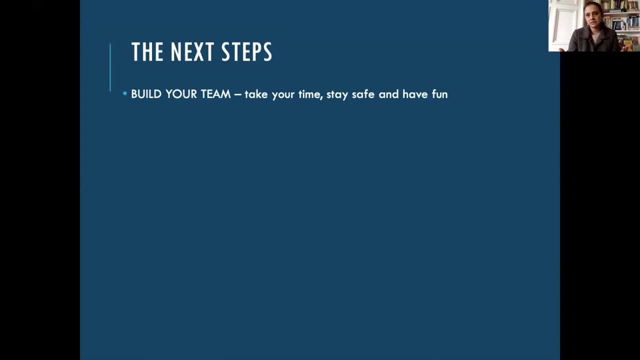 you're still damaging the planet. build your team. have fun building your team, but take your time building your team. let them know you're doing this project. i spoke to our qas pharmacist, who is wonderful. i spoke to the port as well. ahead i, i spoke to everyone. it's really important. you can't 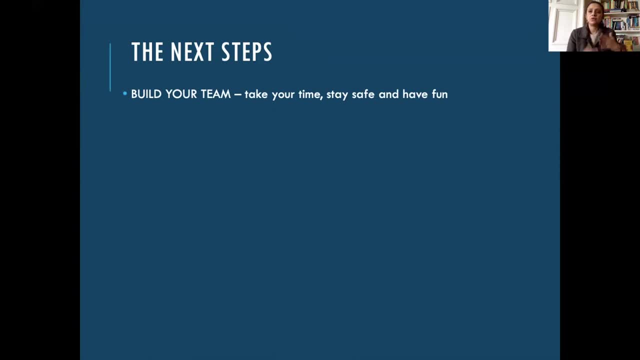 do this alone. it's really important to build your team. we're all under terrific amounts of stress if you're going to gone through a third of the pandemic, so knowing what you're doing and, uh, what you've been able to do is very important. do that and remember that you're under a third of 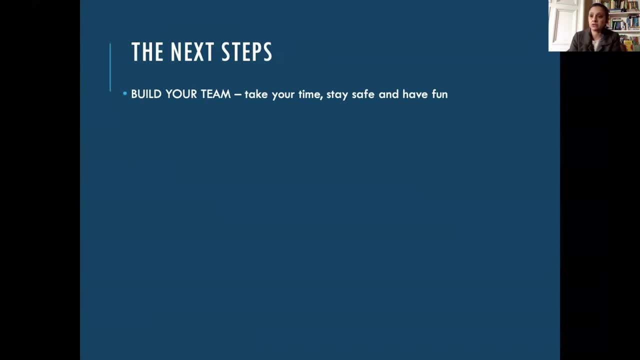 the pandemic, and if you're going to go through it and you don't go through it again, it's not gonna work, okay. so we started one year earlier, in 2018, and we started to work with people who we've worked with for a lot of time and we've had a lot of takeaways and stories and i think 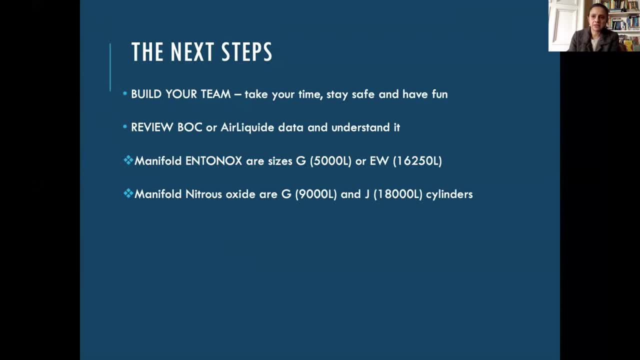 a lot of. it is a place where people really can put their trust in you and your company and who are really positive about you and your business, and it's also a place where people like me and my data against certain calculations- now it's really important to know that nhs scotland and nhs wales. use a gwp of 265 for nitrous oxide based on the current recommendations. you'll see calculators calculating at 310 and 298. they're older calculations, so 265 is the is the current gwp equivalent at the moment, so just bear that in mind. so i put some volumes there of the different 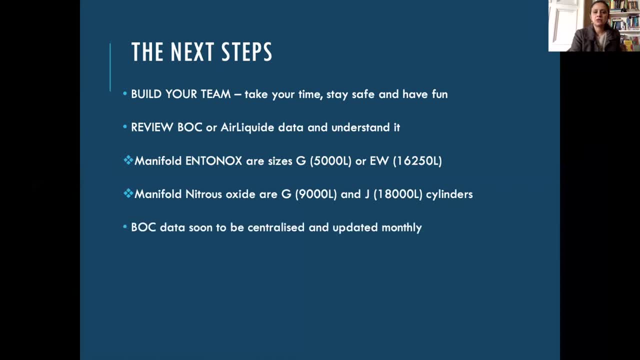 cylinder sizes, so you're aware of them. don't forget, we're also sharing with you. this will be a report that you can get. uh, we'll synthesize. we're serving us and sending out a synthesized report of all of this. so you have, you have a bit of a cheat sheet with, and it contains an audit. 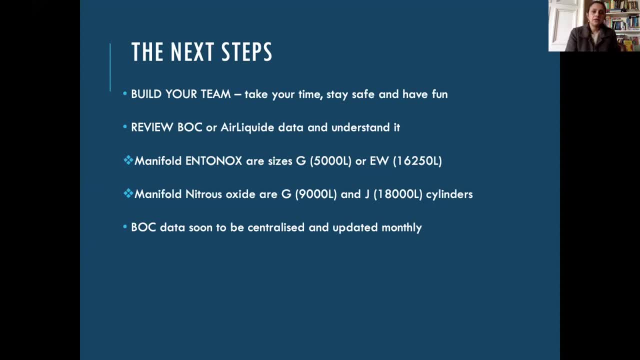 form as well. so you, you have that. we've developed that for you. so the other thing we're doing is we're trying to organize the voc data to be centralized- uh. we're working with the greener nhs to make that happen, uh, which i really hope that will happen soon, and i think some of the greener 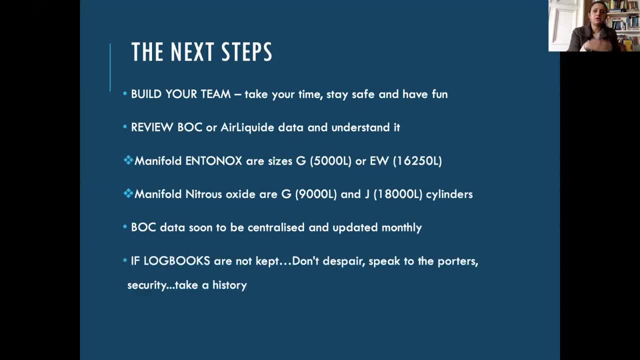 nhs team are on here also. if you find that log books aren't kept- and that's entirely possible, i don't want you to feel freak out or despair- uh, speak to your porters. the other thing is that often when the banks change, it triggers an alarm to the security and they may actually have a log because and if they keep a. 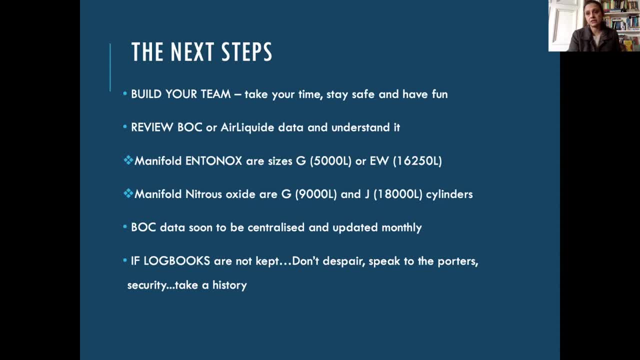 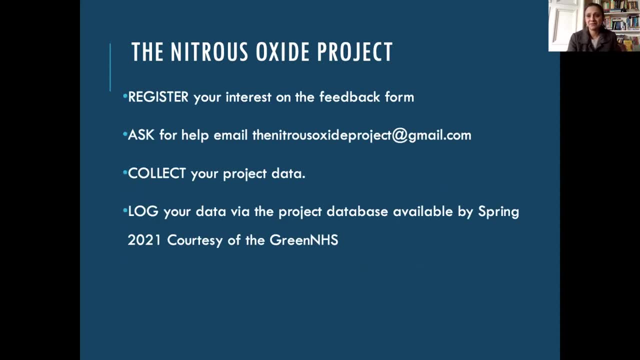 log. that's something you can work with to determine your um, your bank changes. so i hope that all those things help. so this brings us to last page. welcome to the nitrous oxide project. please do register your interest. um, it doesn't oblige you to do the project, but you may know people who would be more. 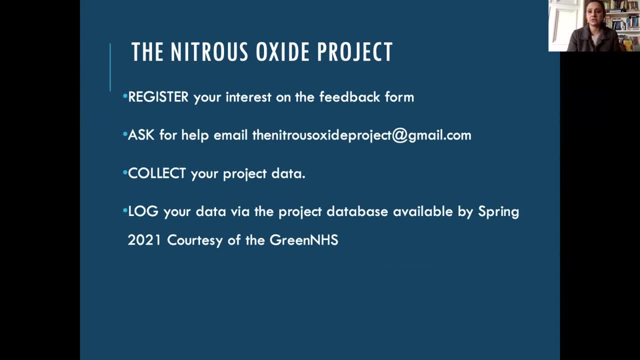 suitable to lead on this project and you can forward on those interests. plus, we can send you all the documents, the audit form and what have you, uh, ask for help. we'd love to talk to you. any of your questions that are that that provide learning, we will anonymize and put on our forum that we're 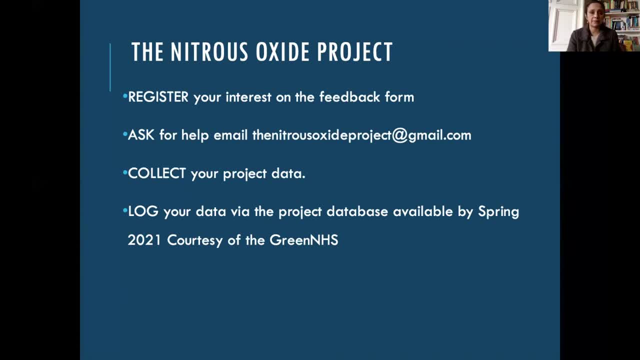 developing. so, um, do ask anything and we're really happy to help start collecting your project data. that'd be amazing. just get started, and we're really happy to help start collecting your project data. that'll be amazing. just get bits of it, take your time with it and pull it together in spring. greener nhs are helping us. 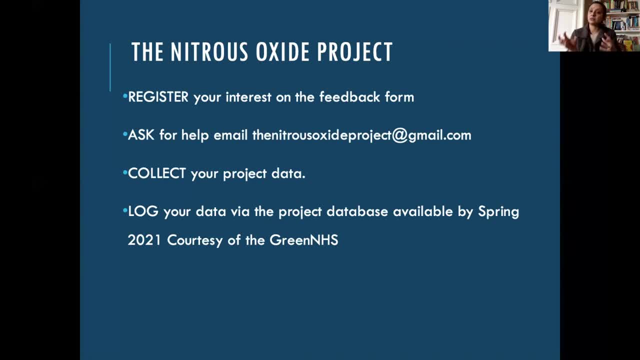 develop a project database so that'll be launched and you'll be able to log your project data on that. now i will finish there. i feel like just talked at you. thank you so much for your time and i'm going to hand it over to chris. thank you, alifia. um, obviously that's not the first time. 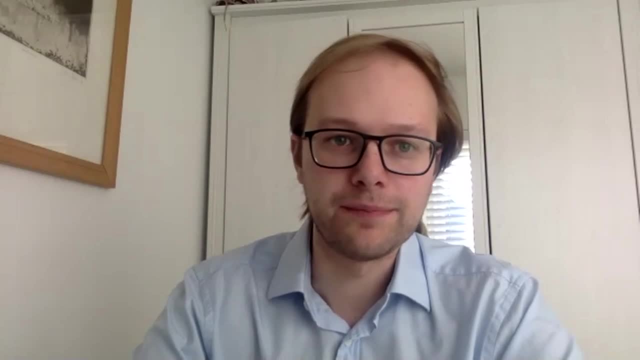 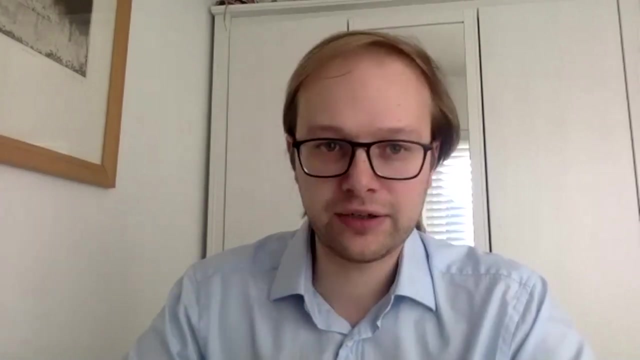 i've heard that talk, but i still find the- um- you know- the data presented shocking about the amount of leaking and hopefully everyone listening feels the same and feels inspired that this is definitely something that can be tackled across the country. um, so yes, i've got some questions. 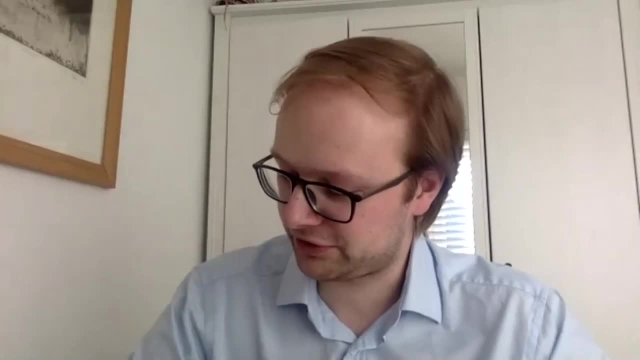 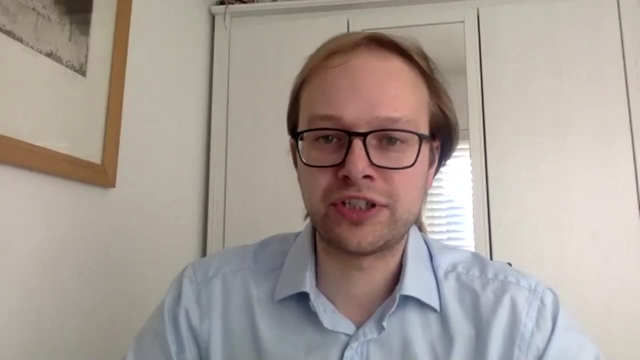 has generated quite a lot of chat, which is great. um alifia, first question for you, if that's right, there's a lot of questions for you here. um what sort of time frame would you suggest? the people looking to do this project would just all give themselves roughly. 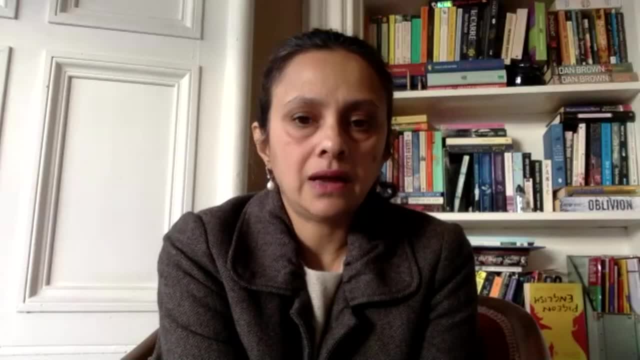 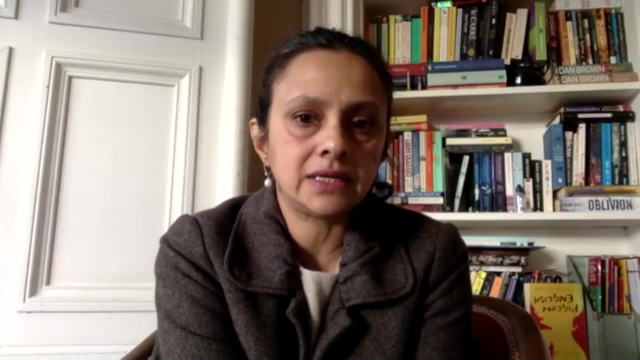 i would allow between three to six months. i would anticipate they won't be able to start till spring because of this new variant, but they can actually start collecting some background data now and they can start building their teams and they should do that. they should just make sure it's a. 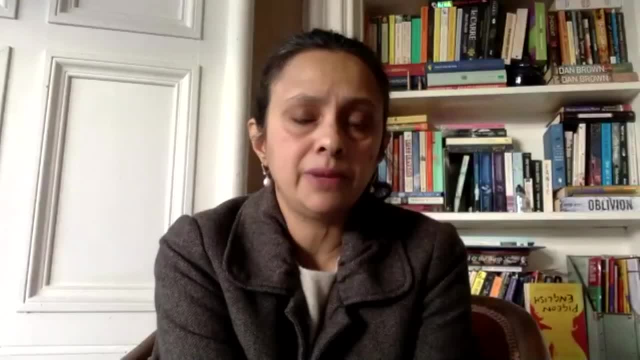 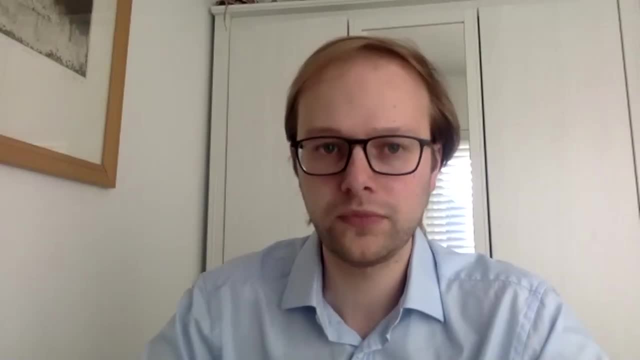 so i think three to six months is a reasonable timeline and not. people shouldn't give themselves too much of a hard time, especially if they don't know some of the players you know. so, um, yeah, three to six months is reasonable, right, and sort of linked to that, what would you say? you know? 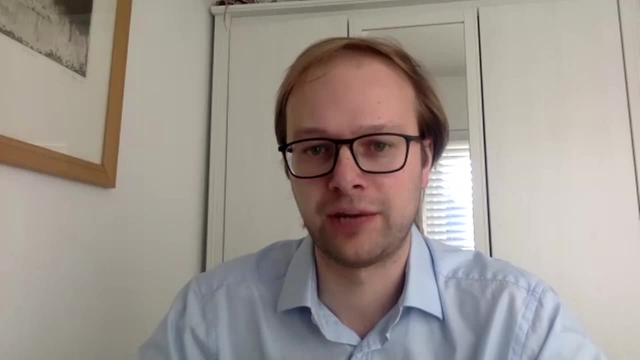 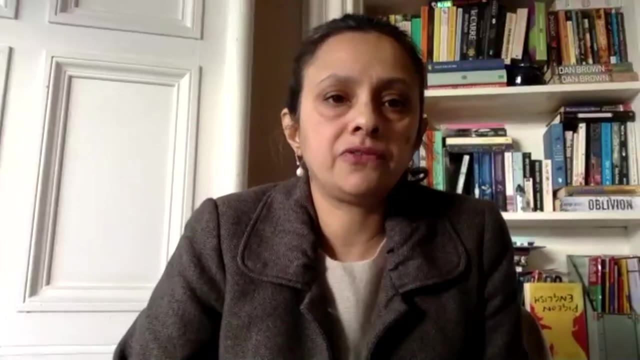 looking back, were your sort of major obstacles that you had to overcome and what are your sort of top tips based on that? yeah, i think um i i was fortunate. i think being a pharmacist is helpful, but i had a really good um support with our qas pharmacist, so that was really helpful. 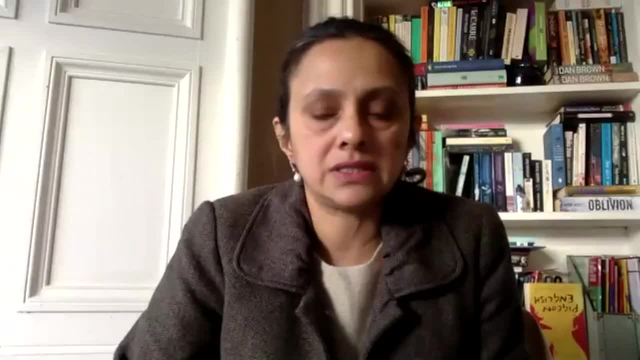 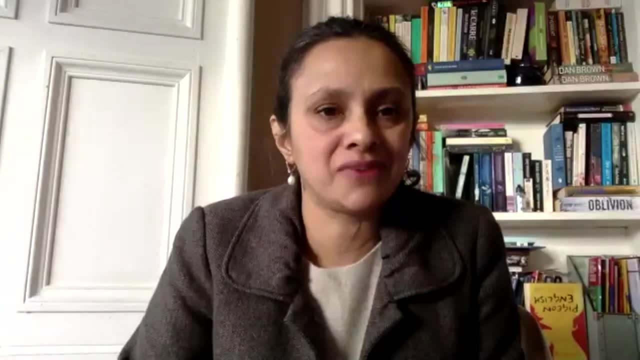 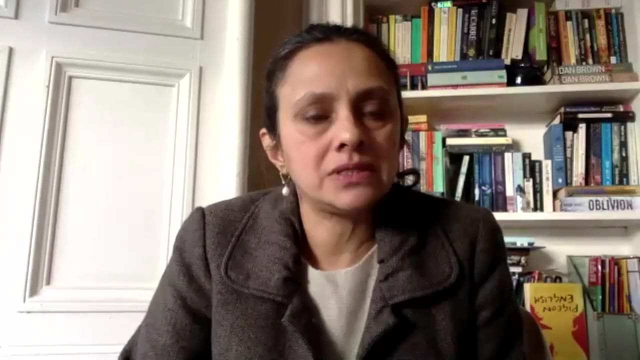 i also spent a lot of time and, yeah, he just told me, speak to this person, speak to that person. it's really helpful. he's put encyclopedic knowledge of who everyone is and what everything does and together. i mean i really spent a lot of time speaking with him. the other thing was, uh, the 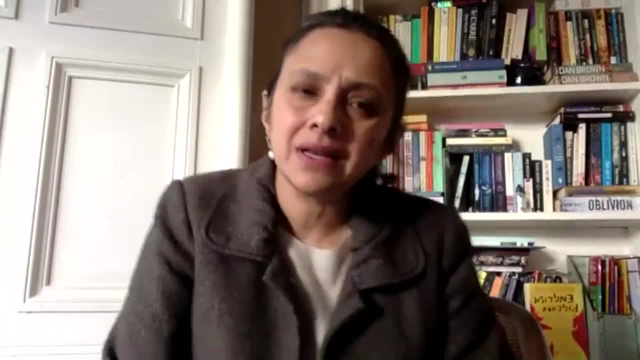 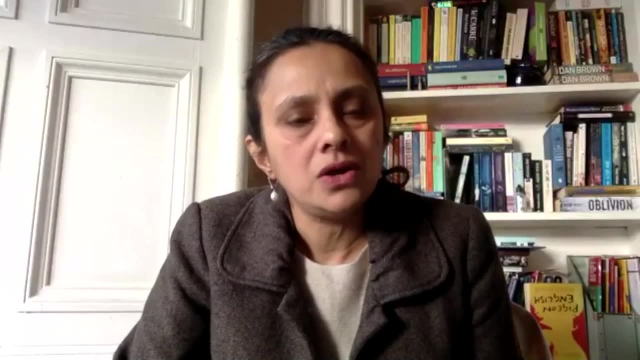 try and try to engage with your medical gas committee. i i was. i was fortunate- fortunate is the strong word- i'd been during this time. i was pulled into the oxygen resilience um work so i actually got to know a lot of key players. so i think, trying to get to know your medical gas. 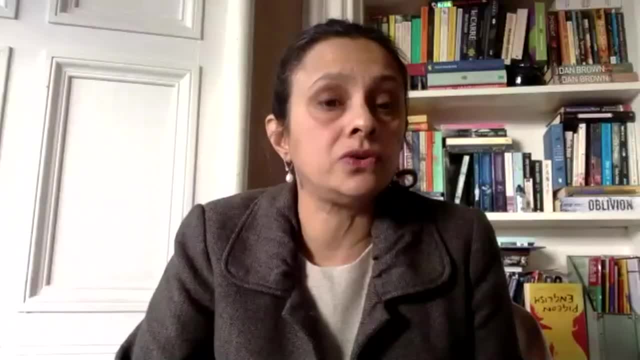 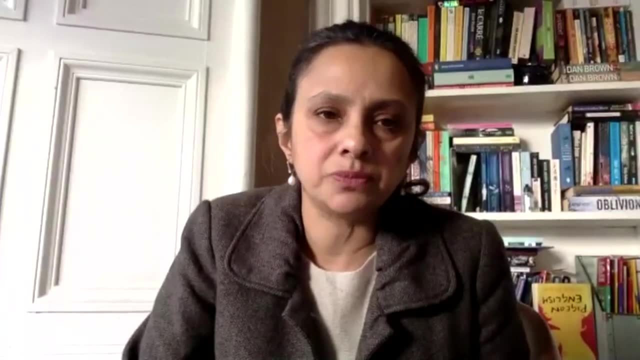 committee. start with your qas pharmacist and start with your director of facilities. they're really, uh, your qas pharmacist. they're really knowledgeable, and they will know the right people to speak to as well, and they tend to be- well, i think they're. mine is very approachable. 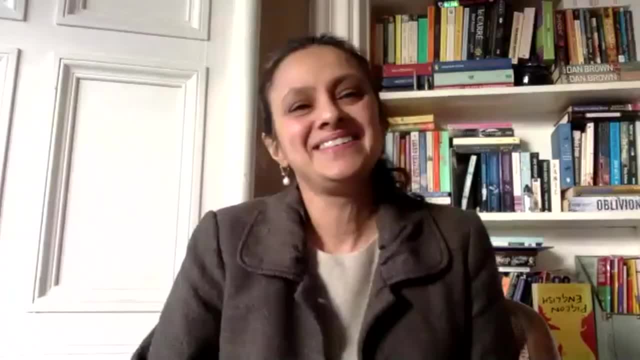 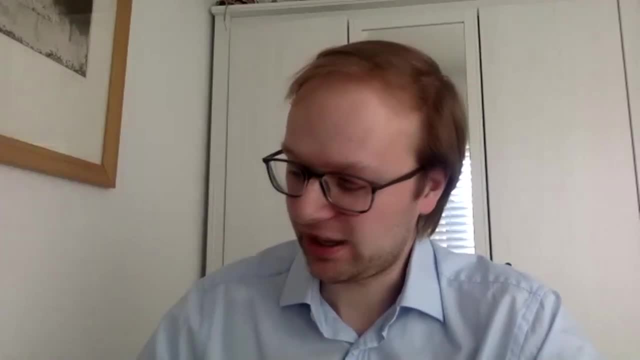 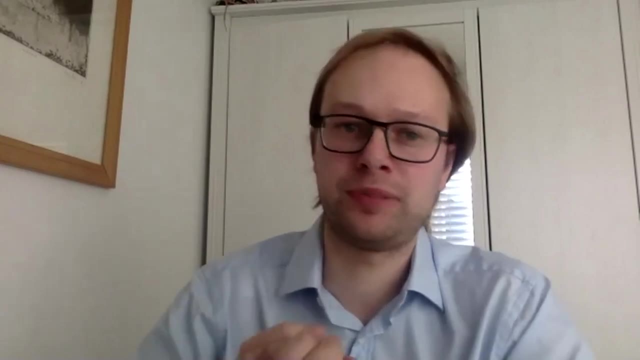 assume, assume, i'm assuming- all our, so your pharmacy department will tell you who your qas pharmacist is. great, good, um, i want a question about dentistry for you, if you don't mind. um what? how can you see this um sort of applying in sort of dental practices or dental hospitals that? 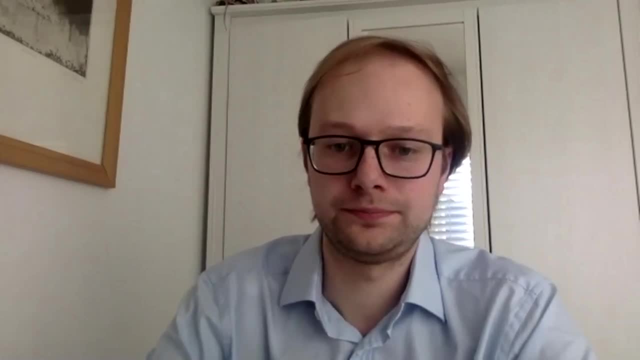 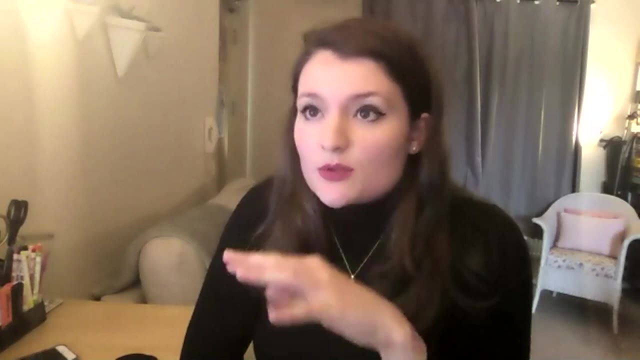 use um nitrous oxide. that's- yeah, that's a really important question. um, you have to look at how they're providing it. i've experienced personally with portable canisters and obviously what we're talking about is piped infrastructure, but i know for a fact that, having started my own investigation, 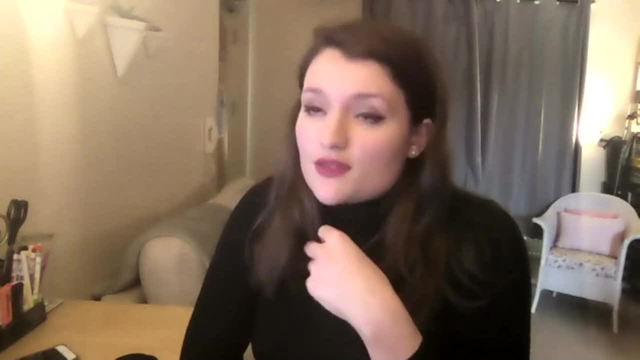 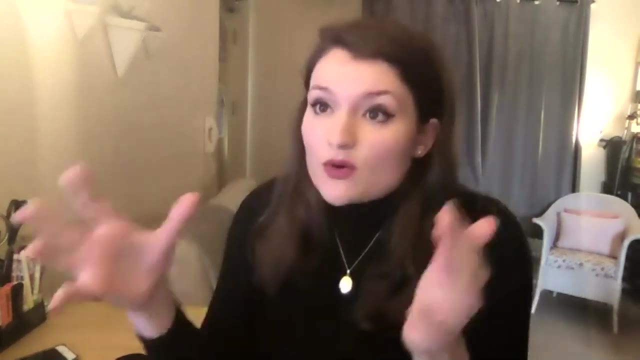 at my current hospital site in cardiff, at the main one, that the dental hospital do does have its own manifold and does have a piped network structure. so even though you're looking at huge quantities of cylinders for different types of manifolds and different specialities, just because it's a dental 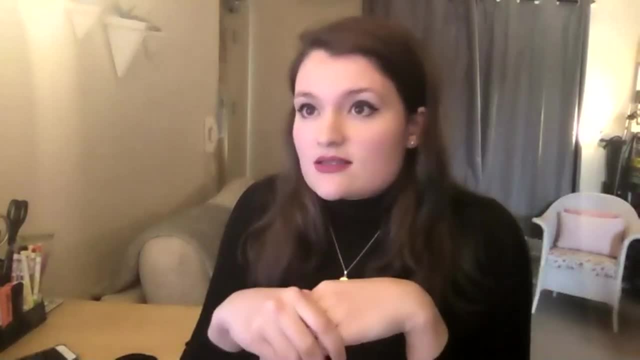 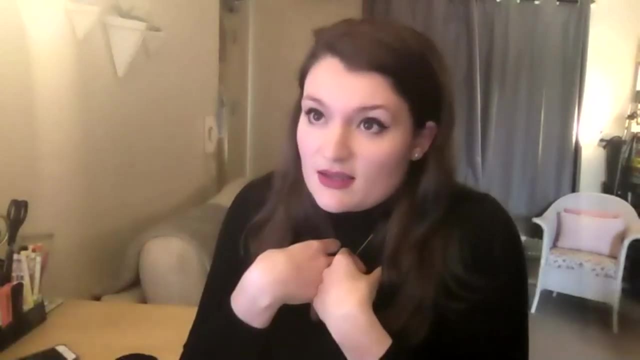 hospital with a small manifold and a small pipe structure doesn't mean it's exempt from leaking. so being a dentist- obviously alifia being a pharmacist has her connections- and being a dentist employed by the health. but i can only imagine that going in i should have some sort of 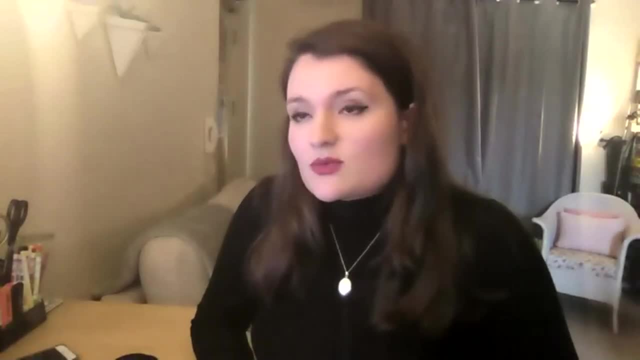 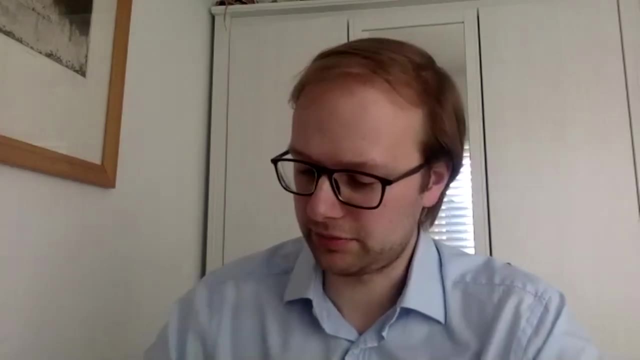 sway in terms of looking at it, but you know it's a small part, but as we keep talking, the small parts add up, so it's it's all about investigating the provision of your own healthcare site. yeah, i absolutely agree that. yes, sort of no matter how big or small your institution is, you know. 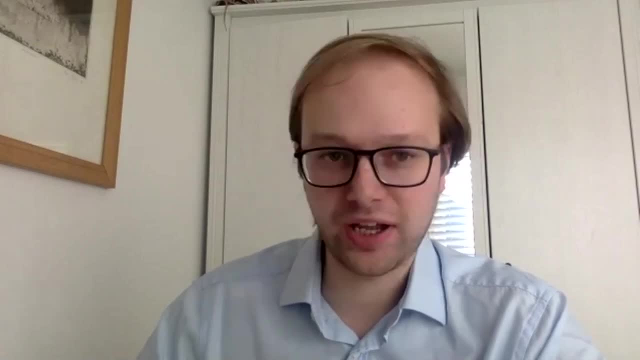 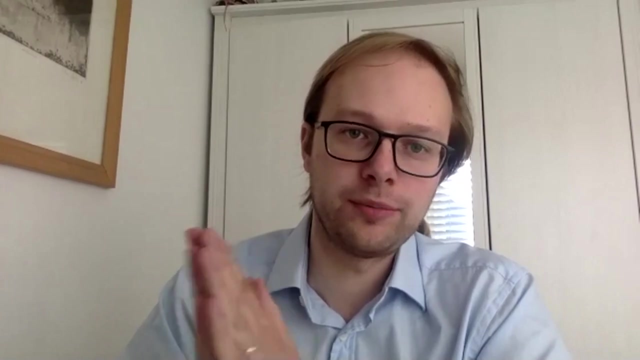 you just don't know how, how leaky it may or may not be. um, i might answer one, if that's all right, on um sort of venting. there's a few people that expressed some sort of shock and surprise about venting. so by that we mean, as alifia said, um, when the cylinders come off the manifold, they're sent. back to boc or whoever owns the cylinders um partially full. they don't get emptied all the way, for various reasons which i won't go into. unfortunately, at the moment that has to then be vented into the atmosphere to empty the cylinder. we've had conversations with boc. 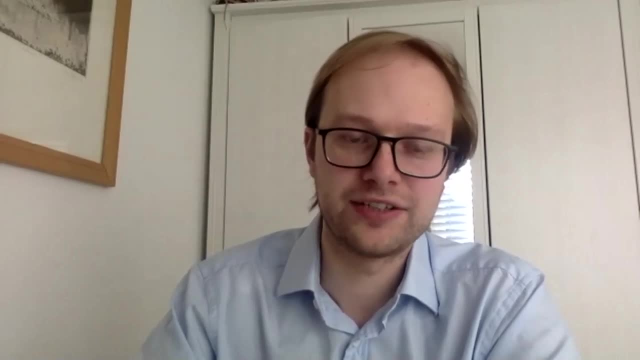 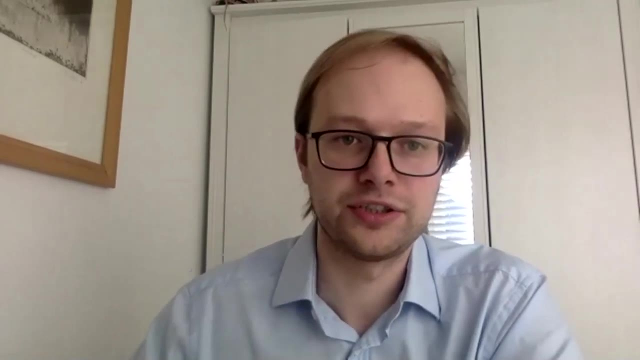 and they are looking into that practice from from their end. so that is something that we'll hopefully continue to discuss with them about whether they can do something to prevent that element of of wastage, because again, that's quite a quantifiable and large amount of. i don't know if you had any other comments about that from our conversations with boc. 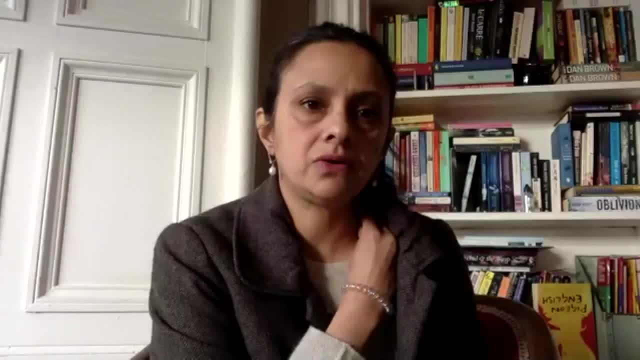 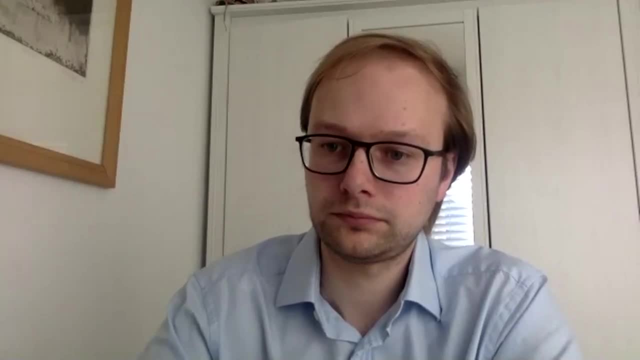 no, i think. no, exactly the same. i, i think boc or uh, i mean to be fair, they've been working very well with us, haven't they? chris? i think they're keen absolutely use their footprint as much as they can and not be part of the problem anymore. so i'm not you know, not that you know, i mean. 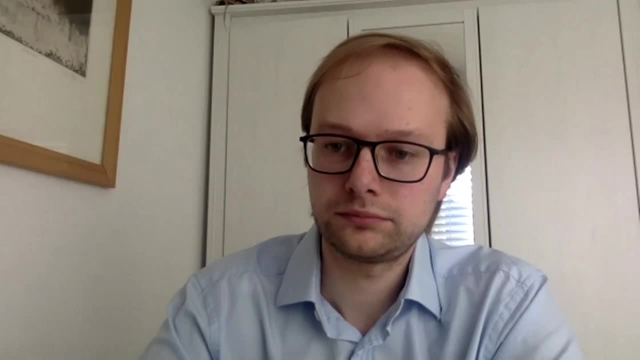 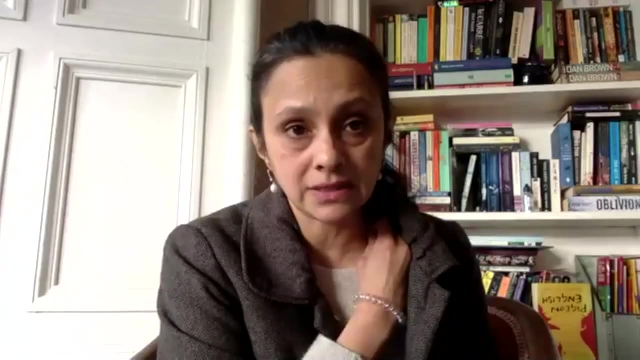 we're all learning, aren't we so, um, they've been to be fair, they've been very cooperative. so i think they're they're looking for the best route to either through legislation, by not allowing that to happen, or by looking at catalytic cracking technology. uh, you know. 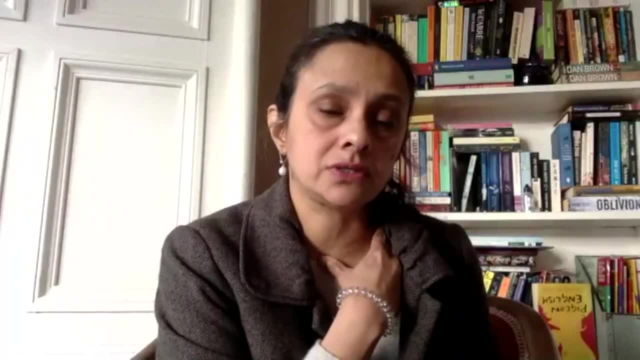 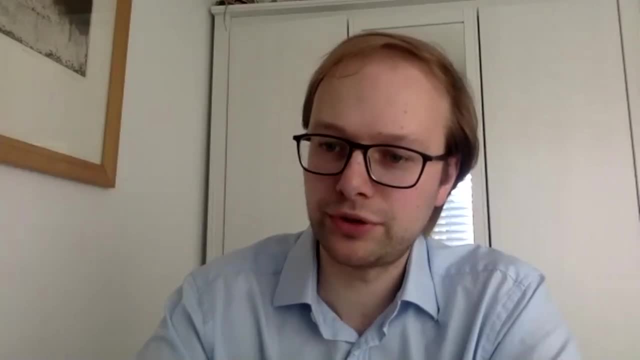 quite frankly, i'd be happy with either, or i just don't want the nitrous oxide just spewing into the atmosphere, you know. so absolutely good um, a good point, which i'm sure everyone is thinking, and as a leafy, you've um said: you know everyone is very busy at the moment. um, so people are. 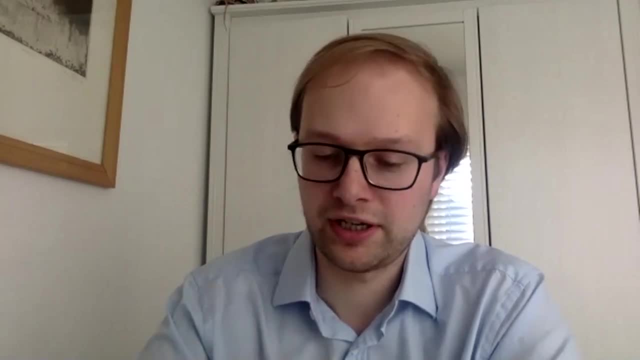 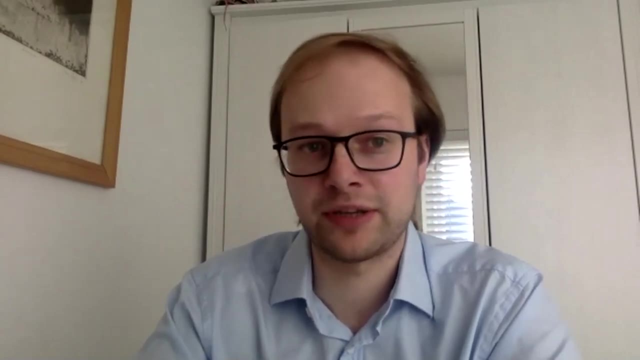 sort of saying: you know time frames. we suggest three to six months. uh, as alicia said, um, you know, we fully expect that some people will have the data sooner, but we fully expect that people will take longer and it it's about taking your time and building the team and being safe, um. 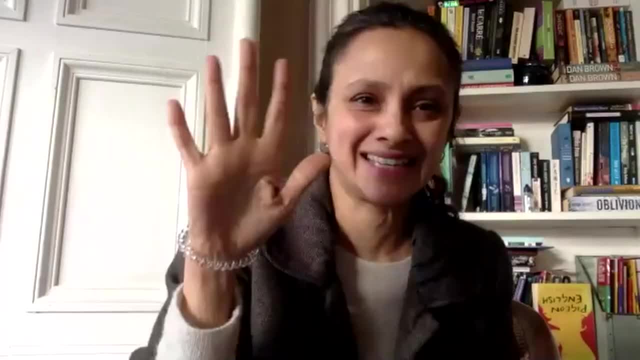 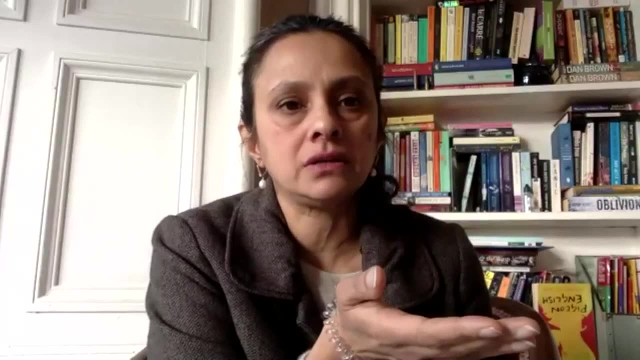 no, no, i just put my hand up as opposed to you can see me, right? um, so i just give you an example this: you may find that the most obvious decision is that, now that you're aware of this, is that you may actually check that, oh actually, we're not actually using nitrous oxide in your division. 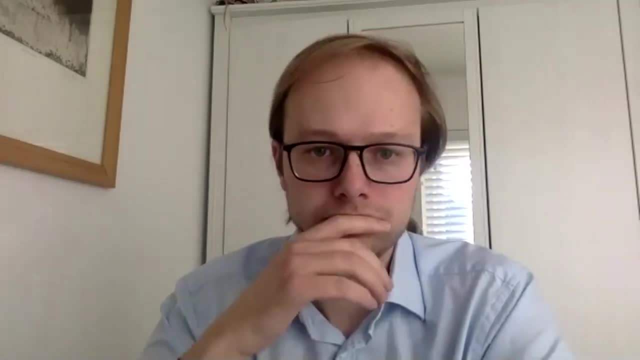 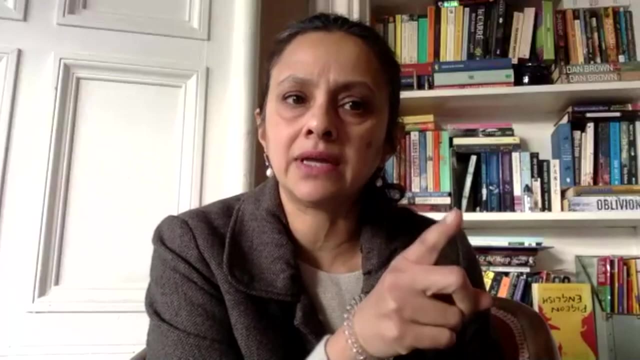 and they give you that information when they don't have it, but then they actually act the same way they do. that's right. so that's why i think that's a good point, because that's the point, for sure. and the other thing that's interesting is the the discritical aspect. i think that you 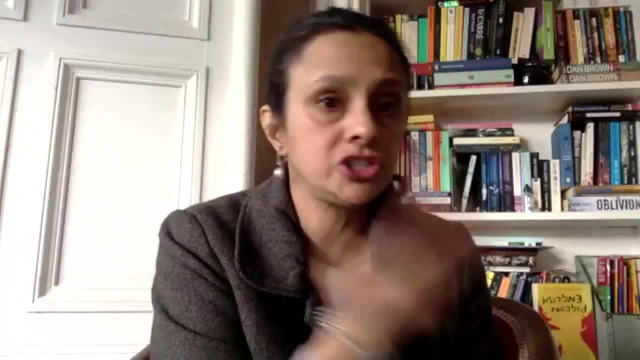 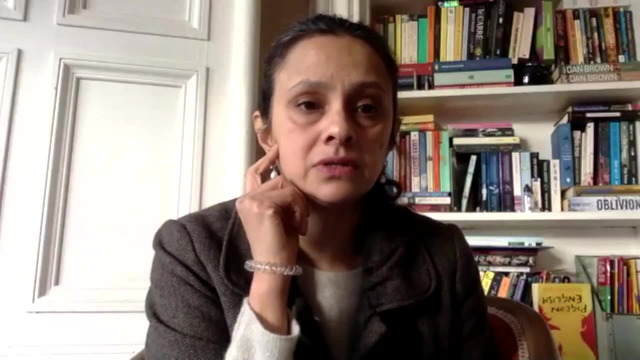 mentioned that, then to me, you know, sometimes you know very it's like, what are the details that you see are very clear, and then you just think, well, how do they solve our problem and how do they solve the problem? what are the technical steps? that's like, do they get it down? 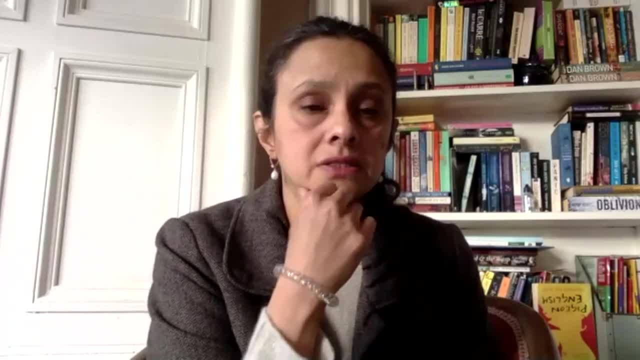 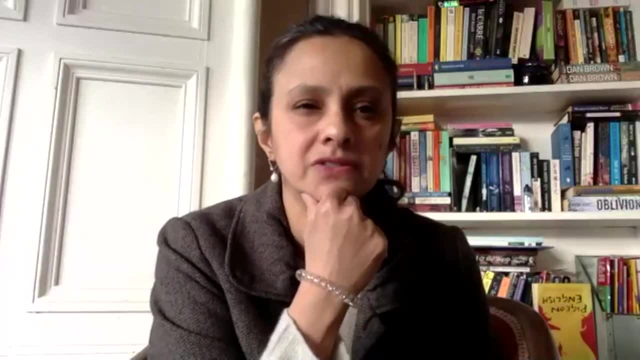 you know, it all depends on what you're doing, and i think that's a really important thing because you've the same in in our site. one, phase two, it we just terminated the manifold, it just there was no, no need for it, and that happened actually very, very quickly. so sometimes the solutions are very quick. 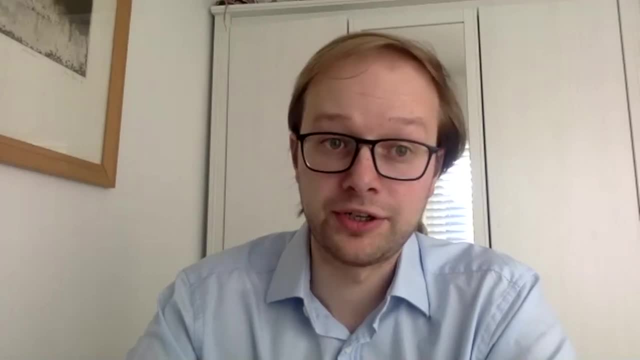 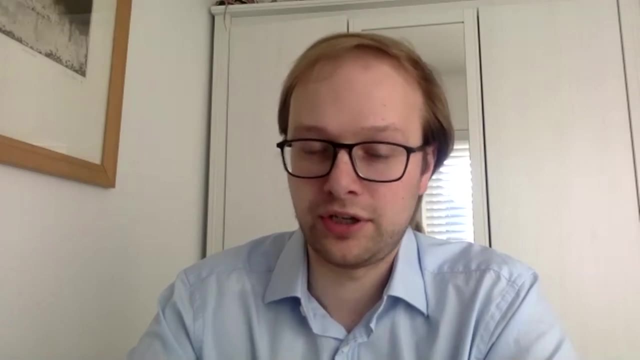 yes, you're quite right. so people have pointed out obviously, uh, sadly, in some places there's no surgery going on at all and everyone is uh critically ill and um, taking up their time, which, um, you know. obviously. you know, then, that your nitrous oxide usage is pretty much zero. so if 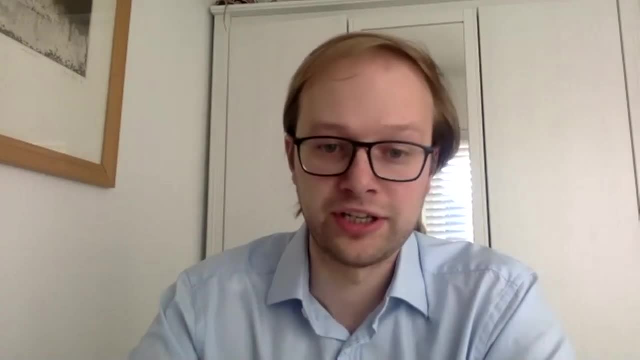 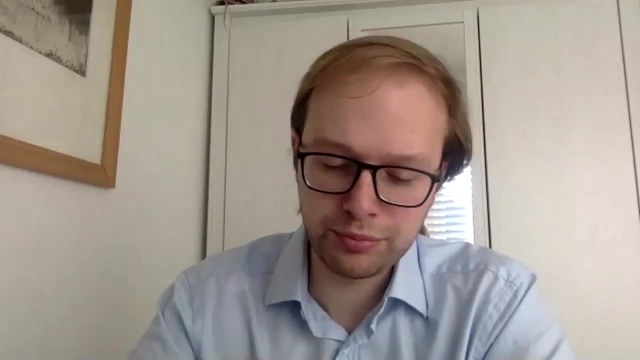 you can then go to your manifold, as leafy was saying, and it's still turning over. you've- you've pretty much already figured out that you've got a leak. so, in a way, um, whilst we appreciate that people's bandwidth is fairly narrow to do other projects, this is not a bad time when. 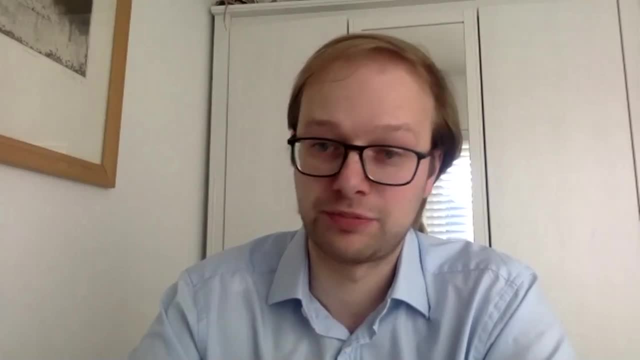 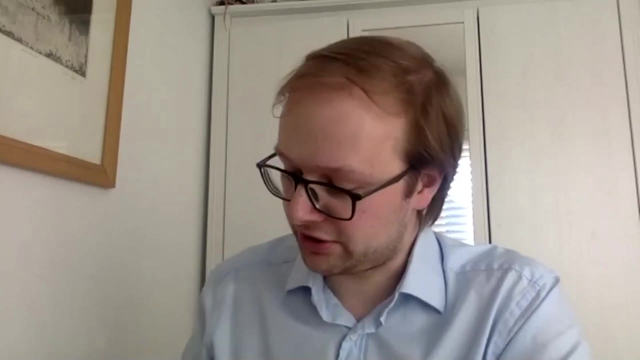 nitrous oxide or sort of general anaesthetic use of all gases is pretty low to look at what your manifold is doing, which is good. um, alifia, a question? um, someone has been very enterprising and already had a question about something that's been doing in the lab for a long time. 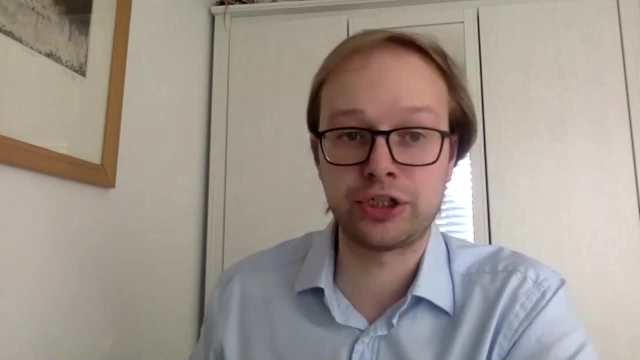 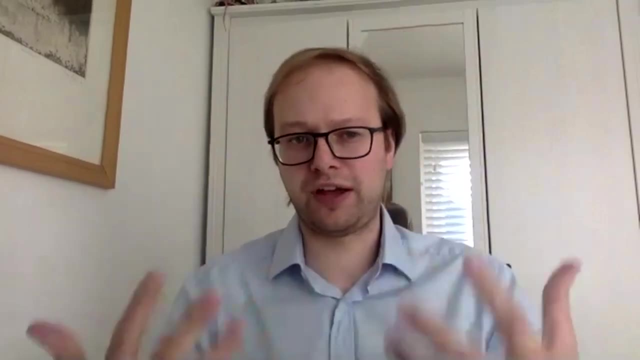 had a chat with estates about sort of this kind of issue and they've been assured by estates there's definitely no leaks in the system. what sort of things would you suggest that they do to kind of to move that forwards? well, i would, i would just initiate the project, if that's the case. 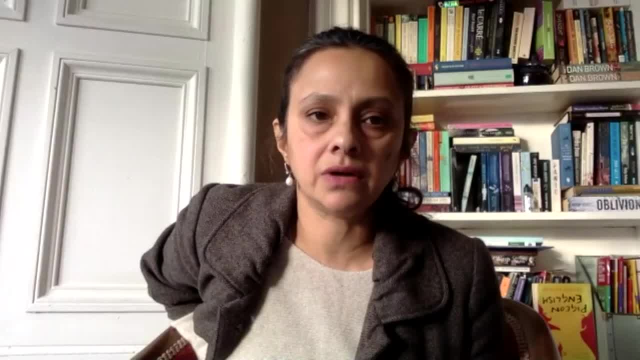 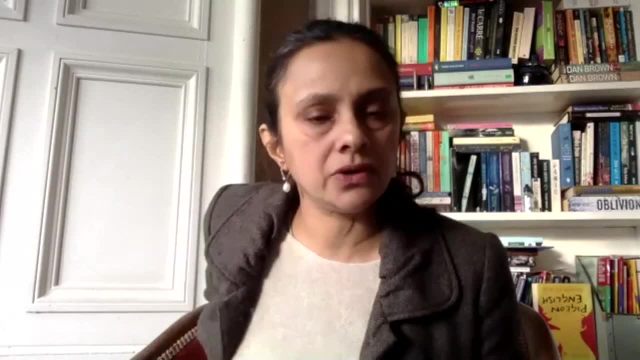 because i was assured that as well, um by an engineer, um, not necessarily one of my own estates engineer, although, to be fair, um that hypothetically it should be a zero, a zero leak system. but i think, practically, we knock pipes, we knock valves, we knock out, we damage things, we leave schrader. valves in. i don't think that's. i don't think that that's true. i think if the manifold, if the manifold isn't tested for leaks routinely, um you, we know. i'll give you an example: uh, one of the manifolds at, sorry, at the rae. they test their manifolds weekly for leaks, which is great, uh. at least three times a year they find a leak right. so you, you know, and at one of the other sites- i don't want to name the sites, but they, uh, they, they weren't doing leak tests and um, you know, it may be all okay, but we know. 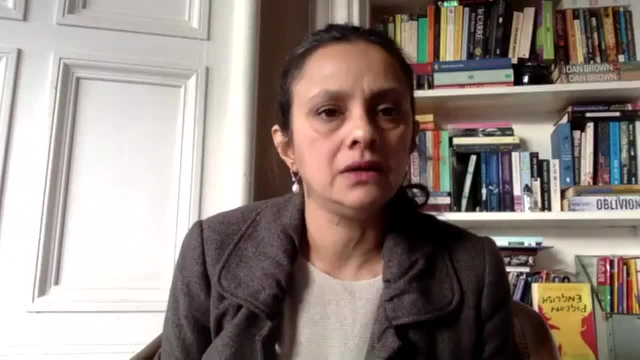 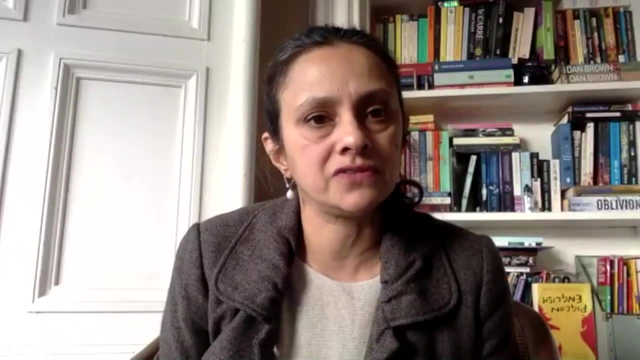 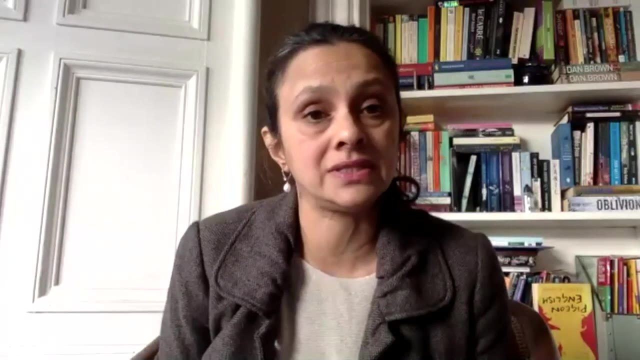 now that a very small leak, a very, very small leak, uh in in what our acceptance is, uh, you know, at our new tolerance level, which is far lower for these sorts of emissions, uh, it can be catastrophic. you know, one liter a minute will they lead to 516 000 liters a year. so that's, it's not not really acceptable. so i think i challenge that. 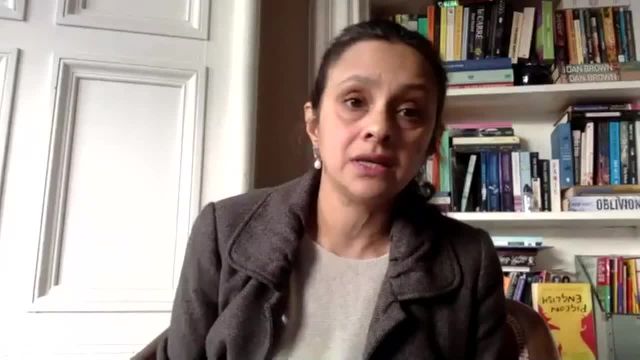 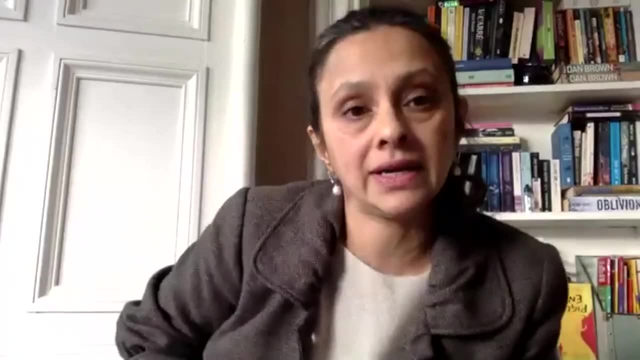 yeah, you will get that, unfortunately, you will get that. but i also get engineers, very, very senior engineers, saying that is, that's impossible. it's a system that will inherently leak and it's top it will tolerate leaks. good, no, i think you're quite right. um, something from the more clinical, uh. 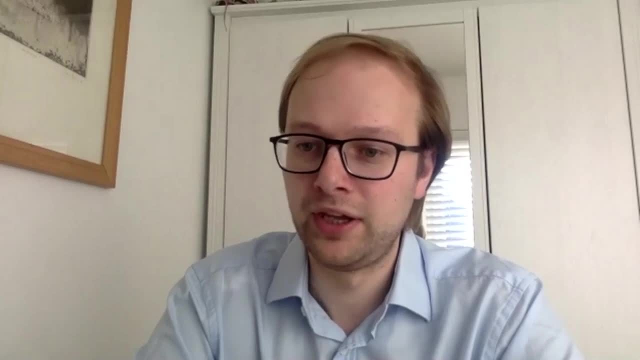 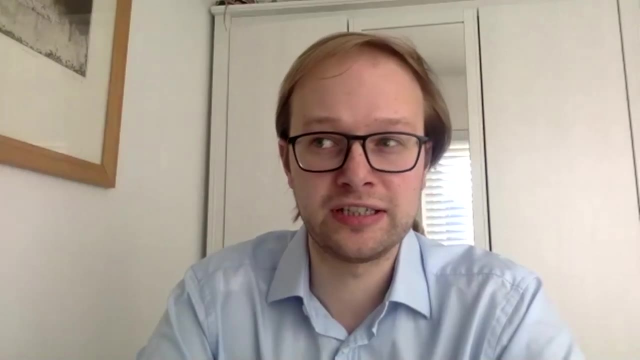 cyber challenge. uh, a few people asking about um, you know, the sort of clinical provision of nitrous oxide? um, and just to reiterate that this very much is is less of a clinical project but more of a sort of um behind the scenes leakage, waste project. um, we still would love people to. 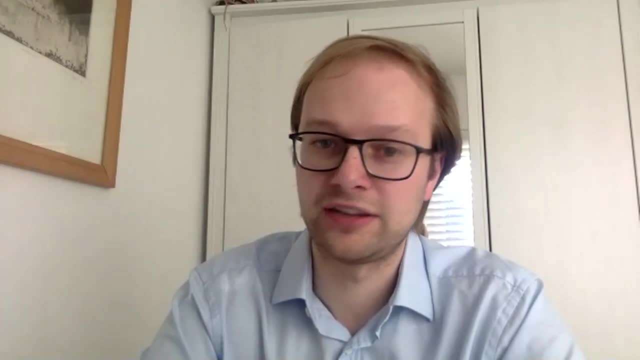 reduce their clinical use and- and a few people have rightly suggested here- um, linking to our suggestion of decommissioning manifolds when you can clinically. that should also be the the thing that people are aiming for, um, and someone suggested, uh, some having it on portable cylinders. 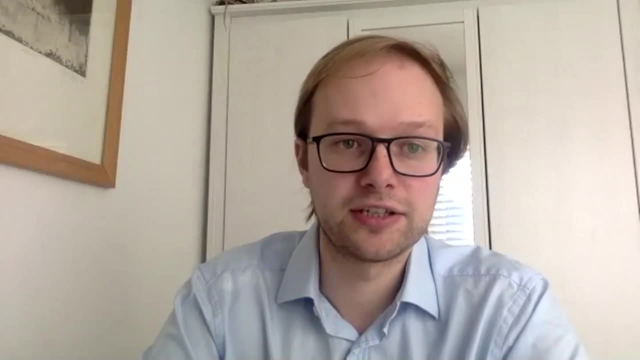 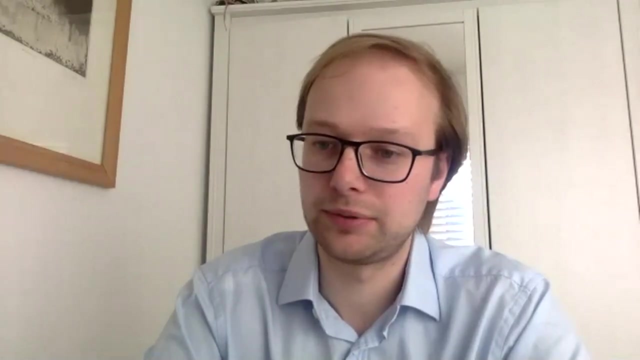 for pediatric anesthesia, and we certainly don't suggest that nitrous oxide doesn't have a clinical role um, and and people do continue to need to use it um appropriately, um, so no, this very much as a sort of uh look at your manifolds, uh kind of leaking type, um project, um, a good question about. 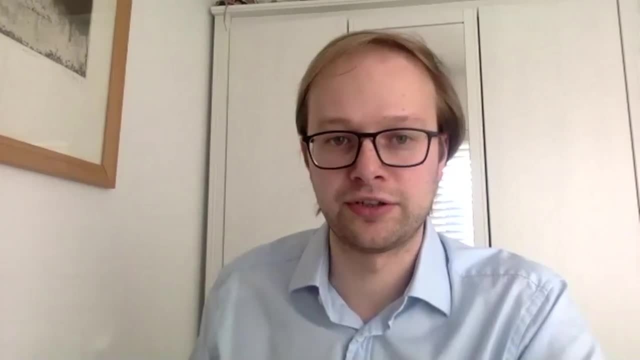 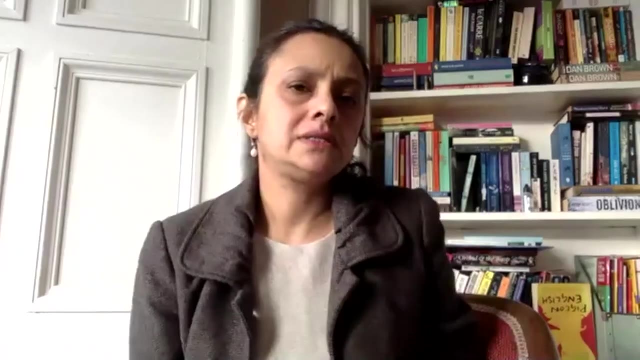 the ambulance service, because they're sort of obviously largest users of entonox. um, and if i think, we had a conversation with boc about entonox and the ambulance service, didn't we? yeah, we did, i i think. so where could we find out where this guy's from? is he from? 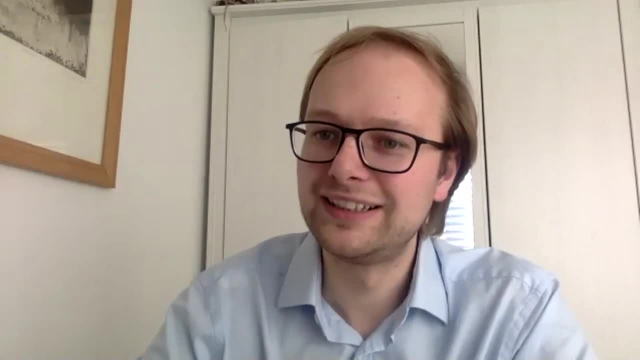 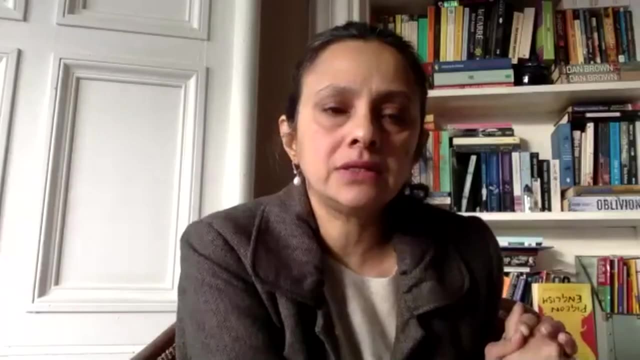 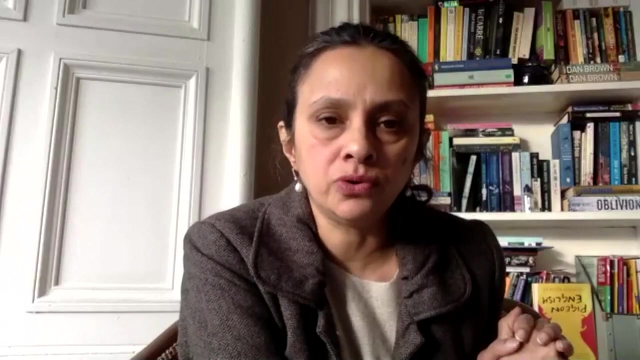 person, i'm not sure, but uh, any any ambulance service people there. so in terms of um in scotland we're now moving towards methoxyflurane, and that's mainly to do with one, that it's more portable, but two, it captures the emissions so the staff aren't. 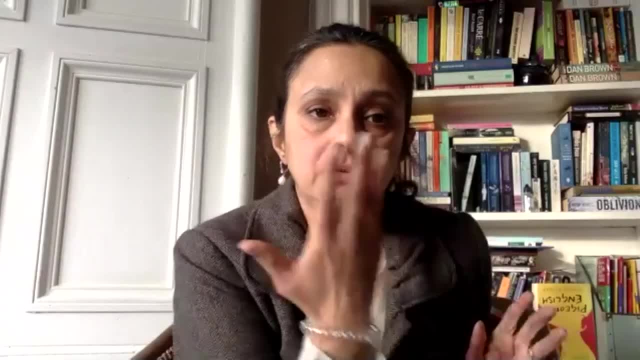 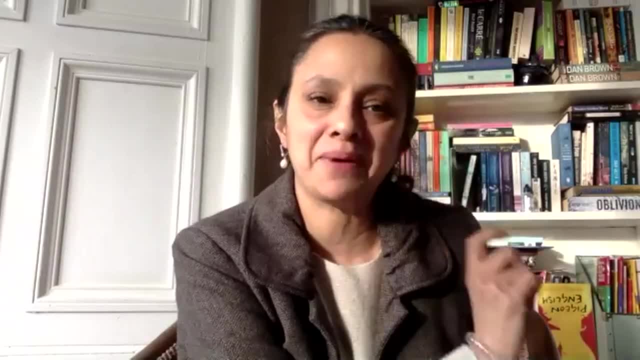 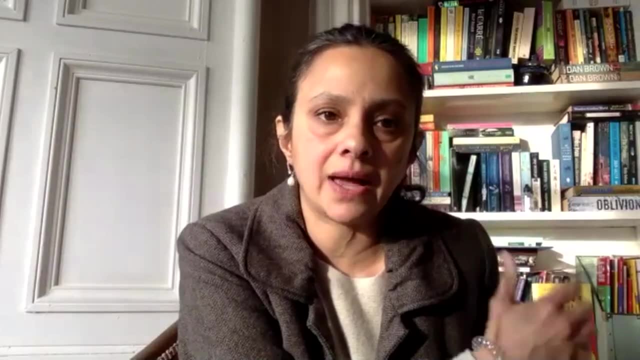 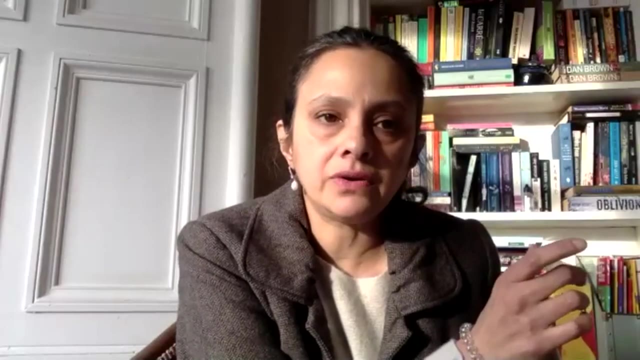 like a vape pen. so it's a bit like a vape pen but it gives. gives sort of roughly 30 minutes to two hours of anesthesia, you know, and anesthesia for sort of ambulatory care. so some ed departments are introducing it and they're introducing it for wound management. uh, i think they're um, in terms of 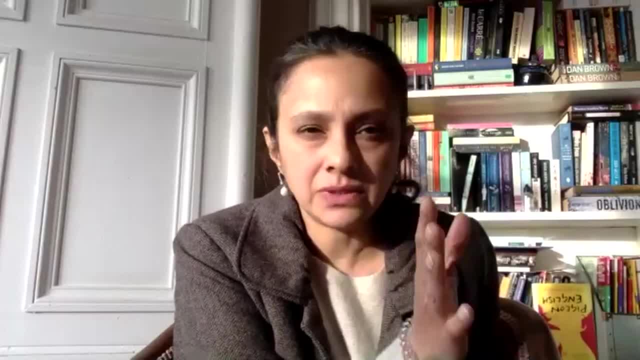 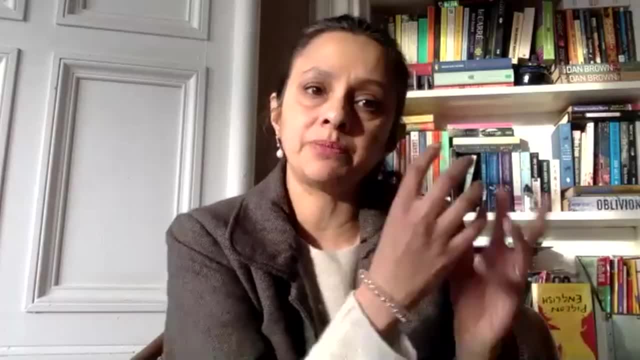 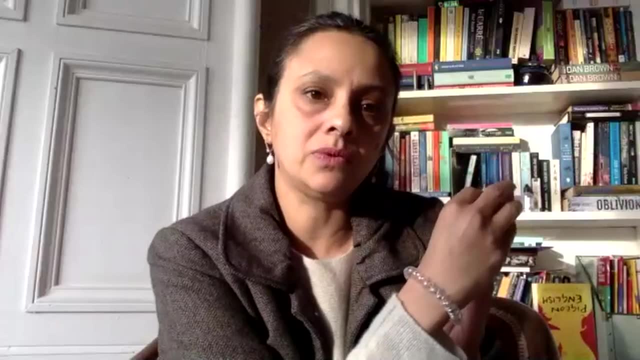 i'm pretty sure it's medic vent uh working on a portable capture canister so as the patient breathes in the um, entonox and nitrous oxide- i think it's entonox you guys use on the ambulance. i'm not sure uh, it will capture it um for for cracking later. so that's an interesting device. so 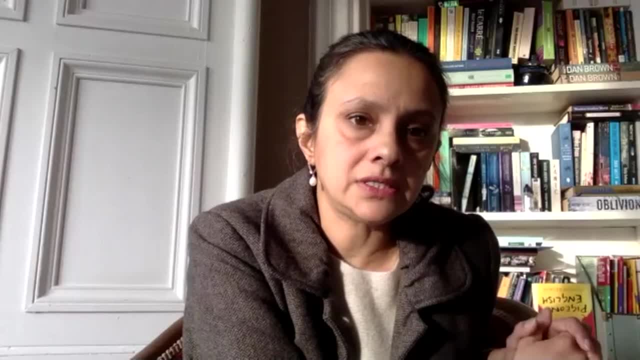 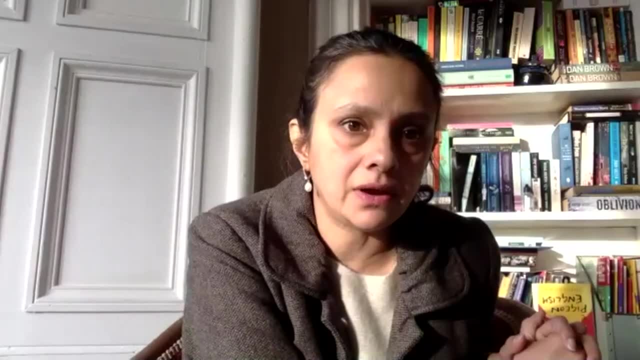 yes, i think. i think there are opportunities to reduce your footprint. uh, certainly. um, this chat could look at methoxyflurane and trialing that within their, their area. i think it's. it's really portable, especially. i know sometimes you guys are going down some really weird. 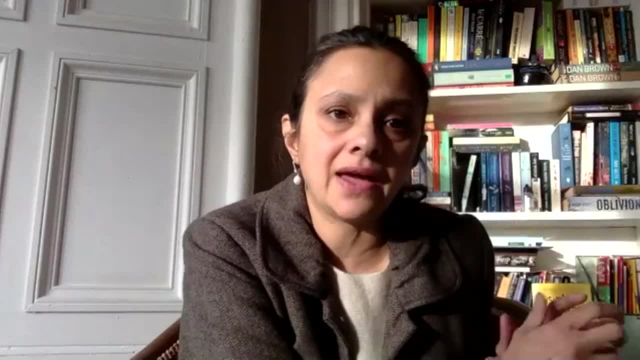 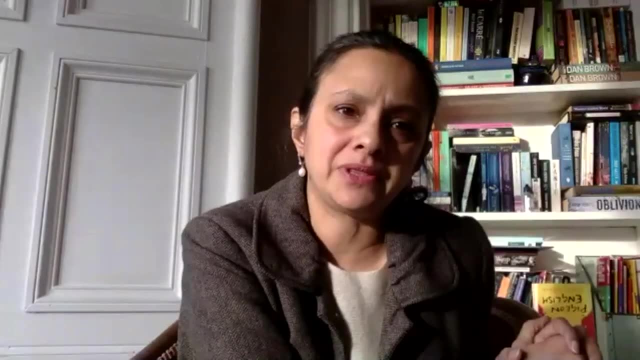 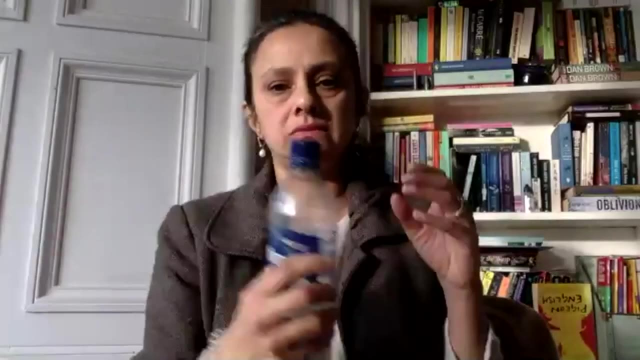 places nooks and crannies to help somebody. so i think having something that can actually fit into a back pocket is useful. um, so i hope that helps. i hope that helps, but there's no good. i think it might be medclair are producing that. um, i think, yes, um, you know, we're in touch with with sort of 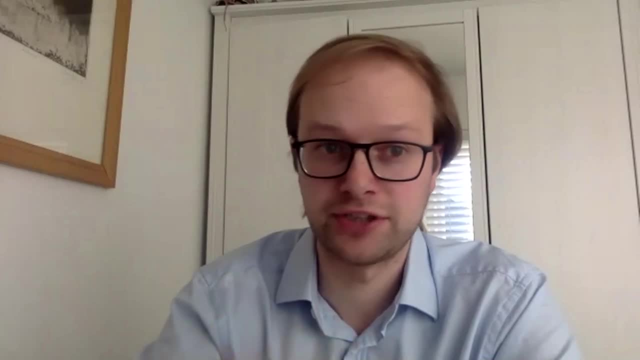 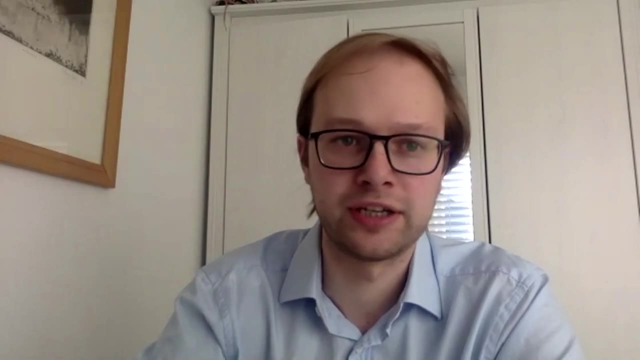 cracking technology, people from um, from an association, beneath this point of view, just to try and explore that. so certainly, the more we can do that um we're going to be working on, that work we do on that, the more information we can give to everyone looking at. 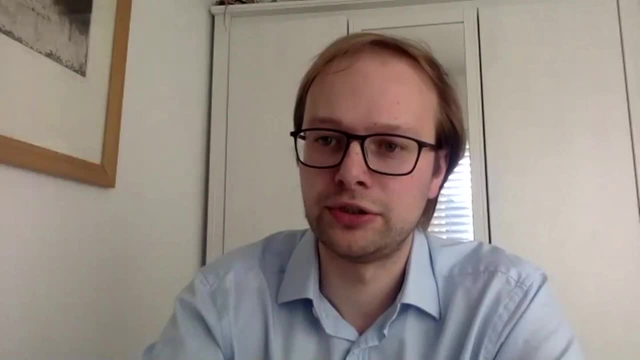 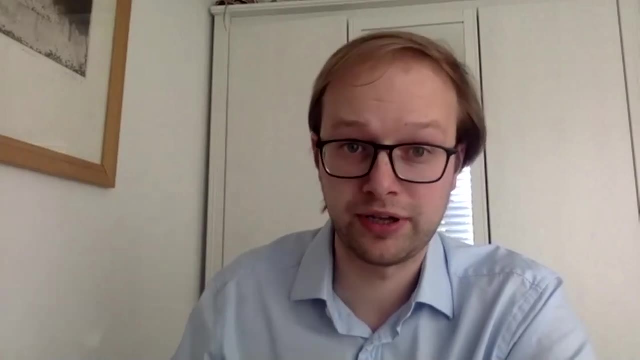 you know that that sort of clinical side of of things as a solution, um excellent, um, i think. maybe last question, if that's all right, and then we'll sort of wrap it up, um, because i'm conscious everyone's on their lunch breaks and i have to be very busy, um. 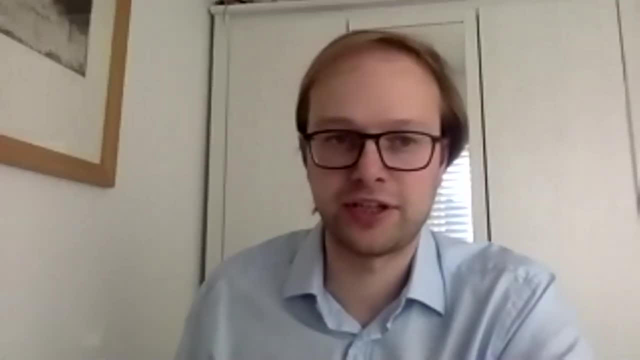 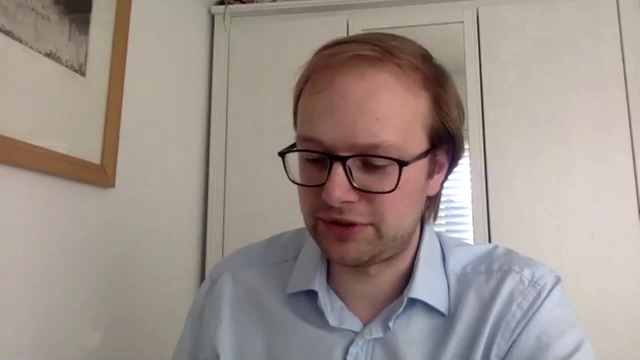 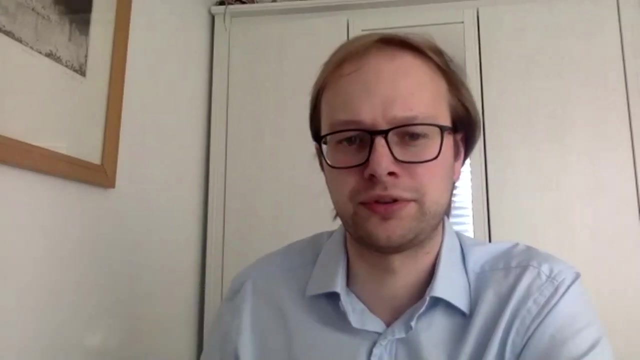 um amaranthi, you mentioned the effects on staff, which i think is a huge issue. um, do you do either have a feel for where these leaks are actually occurring? do you think it's from the manifold room or do you think it's along the pipework and staff are being exposed? what are our thoughts on? 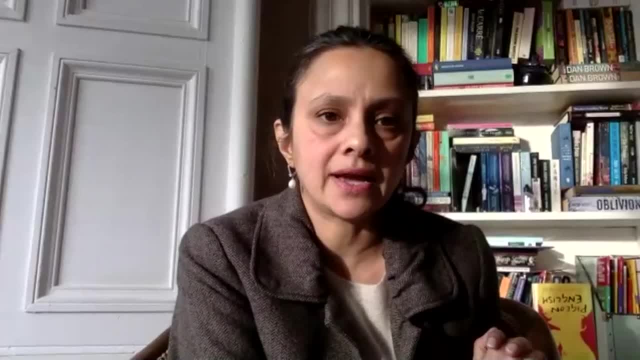 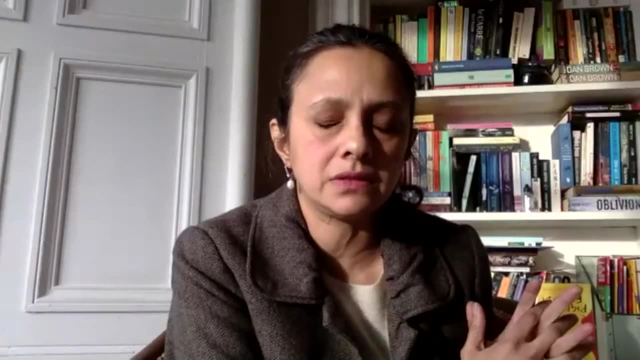 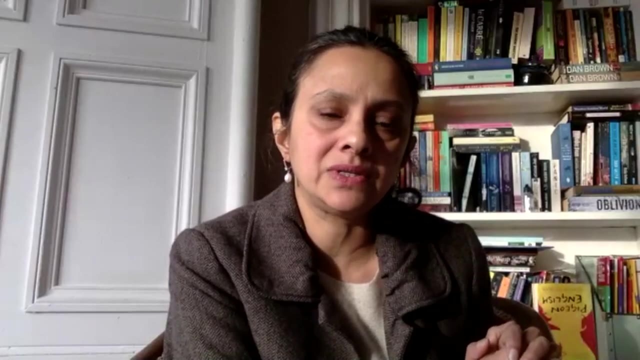 that, yeah, i think i think it's really important not to make an assumption actually where that leak's happening. i think, uh, we, i think, for example, at the site one, the leak was happening in theater, so, um, i'm amazed we didn't get sickness. well, the thing is, i think it was, it was actually a 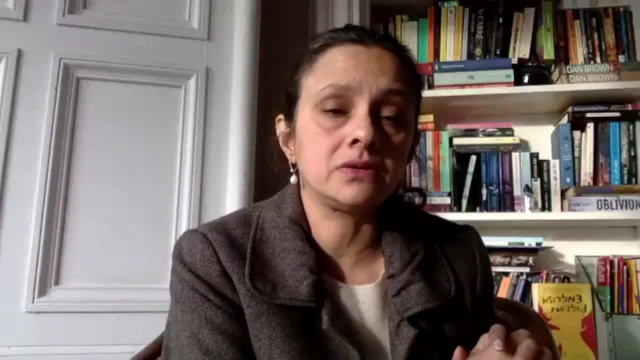 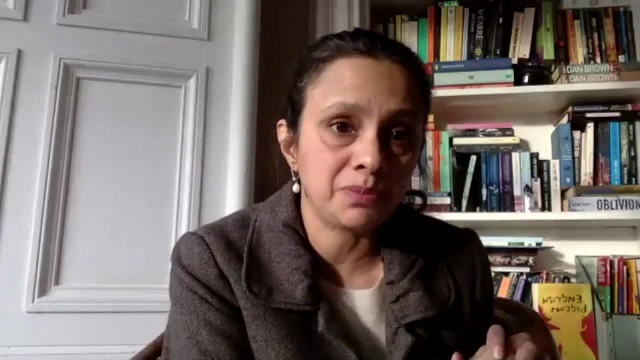 redundant theater. thank goodness, actually it was a redundant theater, so that was a bit of a relief. but the royal infirmary: we don't actually know where that leak is. we have literally kilometers of pipework, kilometers so. but because the usage is so low, we've just taken the decision. we're just 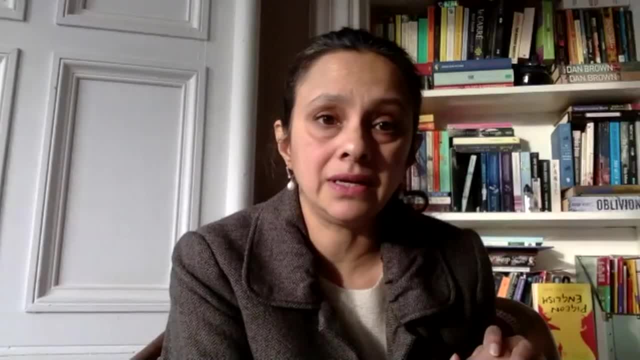 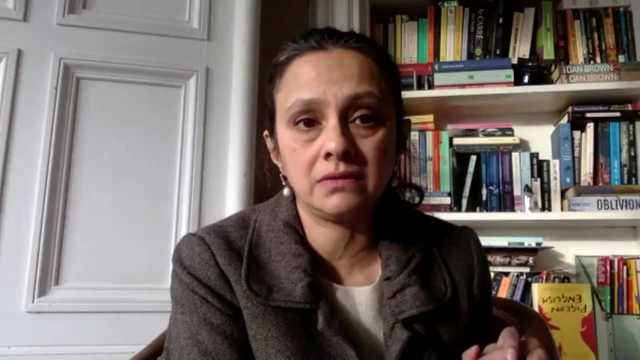 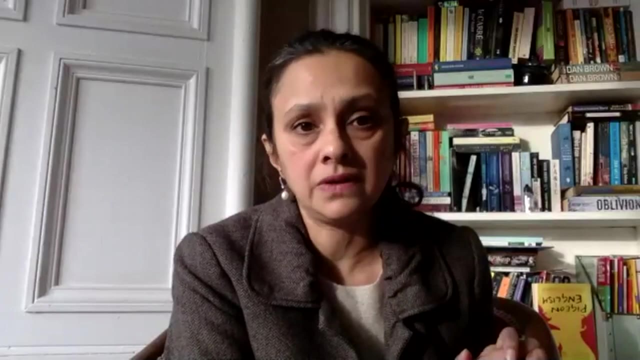 going to close the thing down and i think that's. i think that's completely uh, it's just a pragmatic response by our uh director of anesthesia and i think you know and then and provide a portable solution to that so that we don't have to apply for the areas of low usage till till we work out. 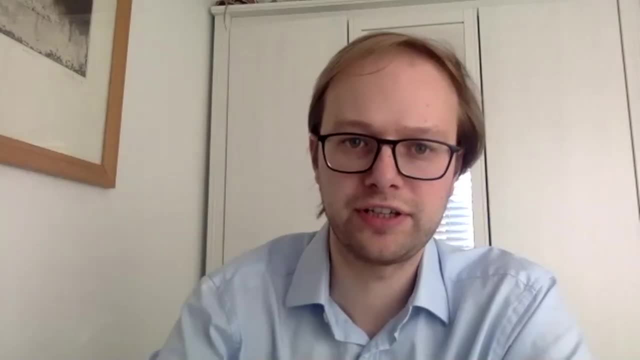 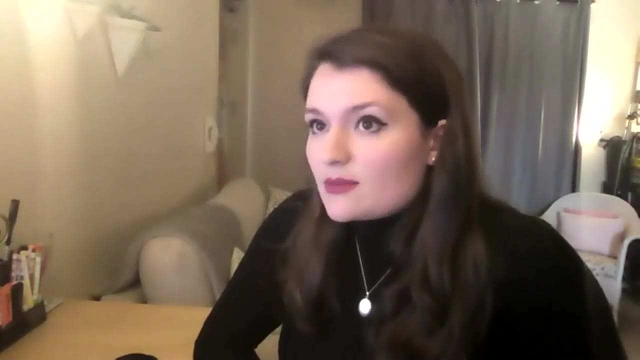 how to get rid of it all together. i think that's perfectly sensible. no, i agree, amanda. did you have any other comments or would you say something along the same lines? um my, my other comments include the, the research, the established evidence that is out there, mostly undertaken in the late. 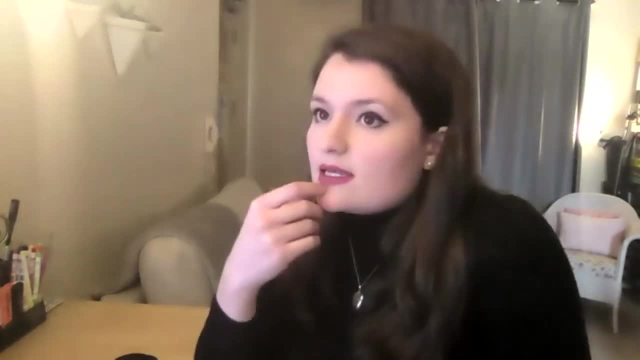 90s, early noughties, around the time where the um 100 parts per million cost regulation was introduced, they actually found that it was the anesthetics recovery room. so, along the what alifi was talking about, the radiology and delivery suites, is where the members of staff. 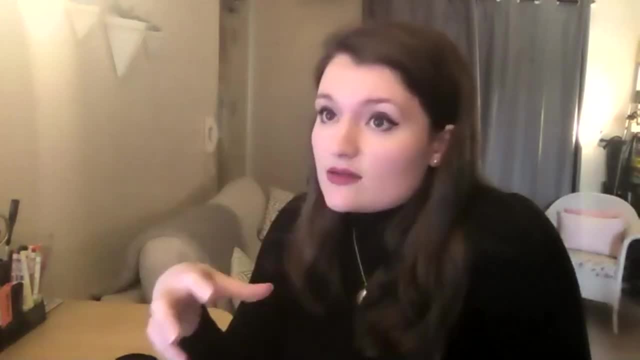 were being picked up as having either high concentrations in their exhaled breath, in their urine samples. and then the most concerning is that theater personnel were more likely to have a higher chronic nitrous oxide blood concentration following on a shift or even beyond having a shift. and obviously, dental personnel without correct scavenging. 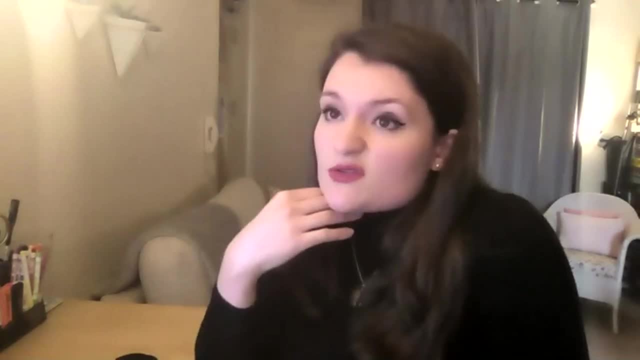 are more likely to be around environments where the nitrous oxide is just sitting there. so there are certain pockets, but those are the only people we've tested. you know those are the only ones who have been actively sought out. so you know the jury's out on that one. like alethea said, 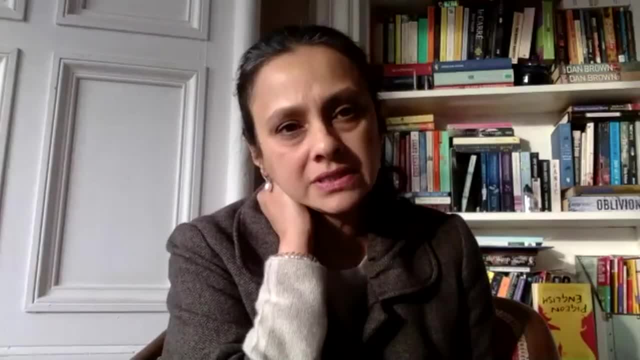 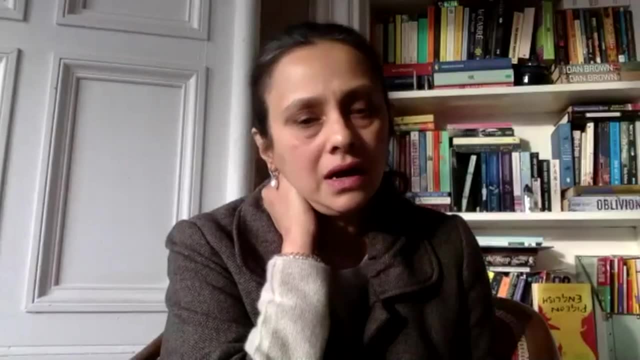 i have to admit i'm i'm very concerned for midwifery staff. i think we don't have active scavenging in our labor units um at one of our major sites. i i find that quite shocking and worrying. um, i'm not going to pretend, i i think there. you know there's some studies done in the 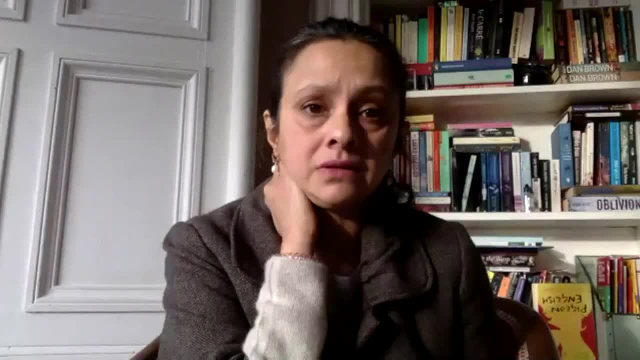 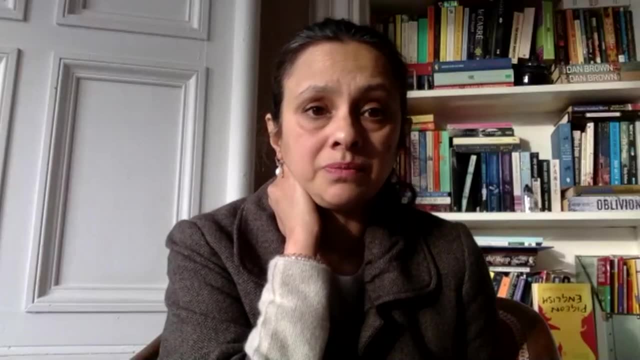 midwifery that have shown that there's a very high percentage of midwifery staff in the midwifery that have been affected by the impact on women at childbearing age. and you know the thing: a midwife might have their own fertility impacted or often suffering from chronic anemias that aren't 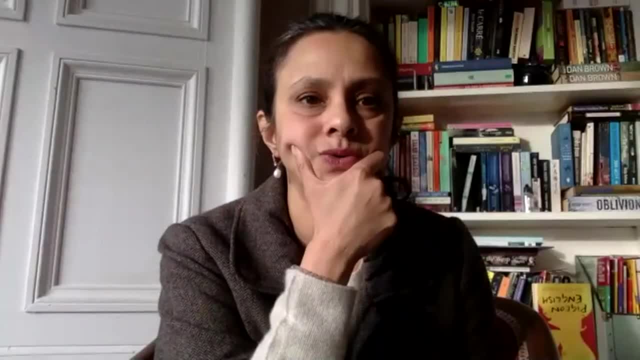 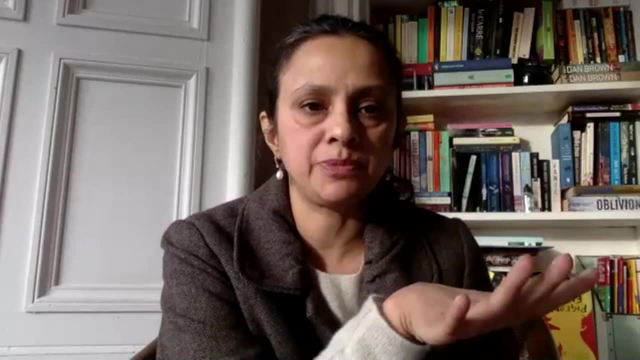 necessarily associated with their professional- you know- work exposures. so i think there's some really interesting. you know something: we've been talking about some interesting work that's being done on this. um, i have been done on it. so, yeah, i think, yeah, i have no doubt that. 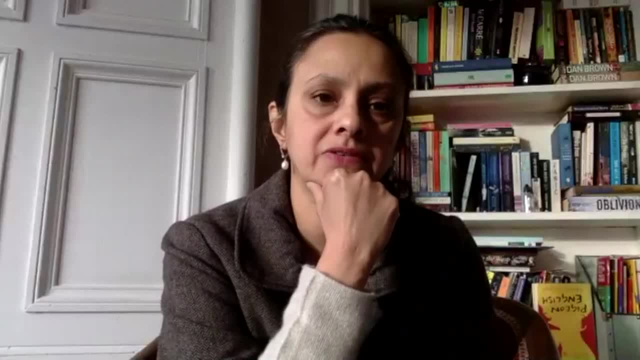 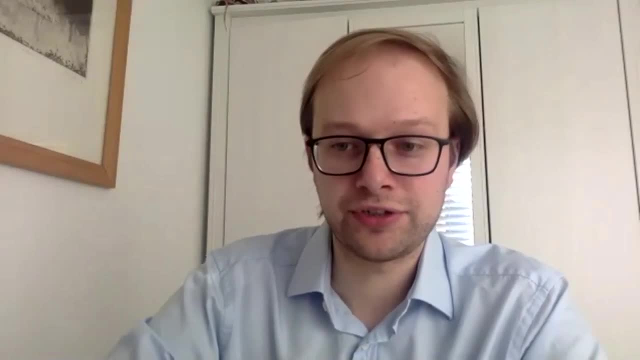 there's a lot of work to be done on this and and i, yeah, we need to be, we need to be more cognizant of that, really. no, absolutely, very, very true. um, lovely, well, i will end the questions there. i'm sorry to everyone who's asked lots of other questions that we haven't got time to answer. 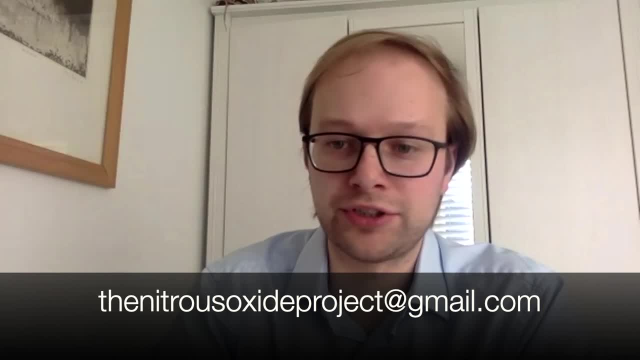 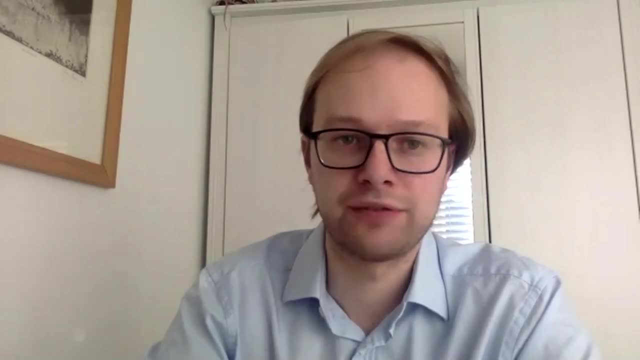 them. please do um. email us um about anything you want to check uh. just to reiterate again, we've got a really great package of um you know, like a how-to guide, with uh resources available. so anyone wanting to do any kind of work on this project um, we'll have our full support and help um and we'll sort of 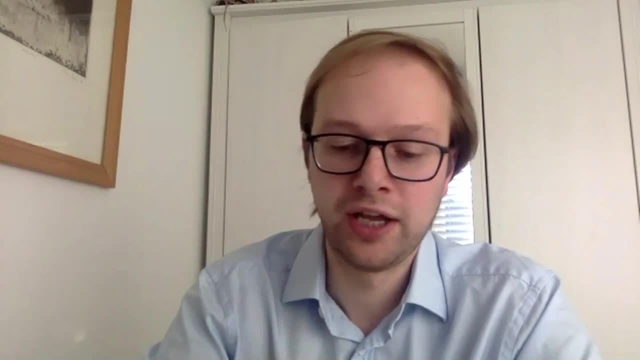 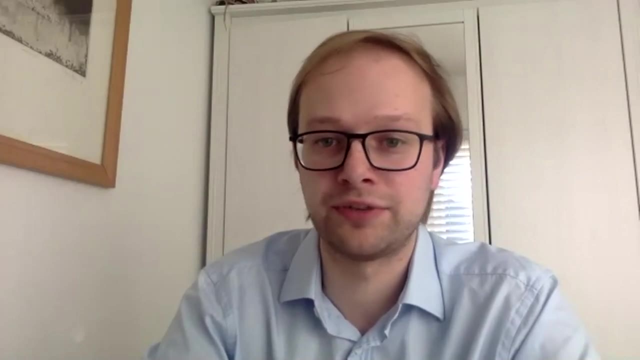 continue to evolve uh together as we sort of all go along. i've no doubt that other places doing this project will um have their own issues that perhaps um we haven't come across in the places we've done it so far. um. i'm going to pass it on to amarantha now to make a few closing remarks, so